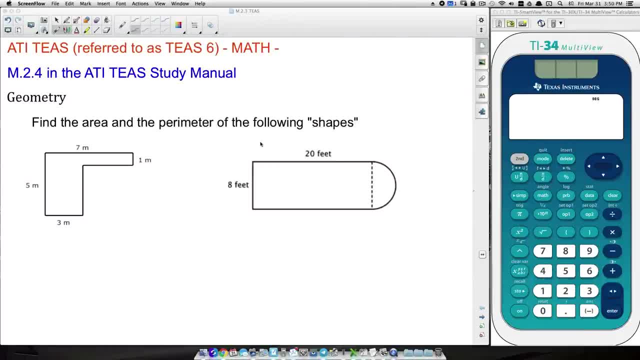 All right. in this video we're going to look at goal M.2.4 in the ATIT study manual, and this goal is focusing solely on geometry. If you're following along in the ATIT study manual, you will notice that there are several shapes, parallelograms, rhombus or rhombi. That's how. 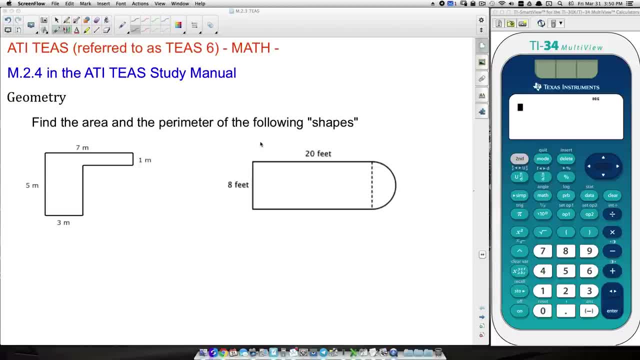 you say them in plural, or rhombi, I don't think. don't quote me on this, but my personal opinion is I don't think you need to know all those formulas by heart. There are some that you want to be familiar with, such as rectangles, circles and triangles, and those are going to be the ones. 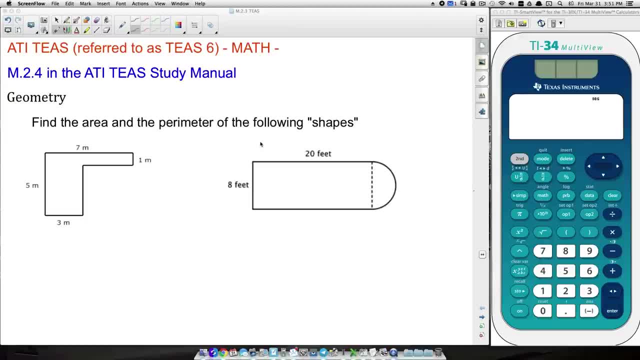 that I cover here To play it safe. if you can memorize them all, great, but the ones that I think you really need to know are rectangles, circles and triangles, and we're going to look at four examples in this video: These two, or these two here, and then this one and this one, right? 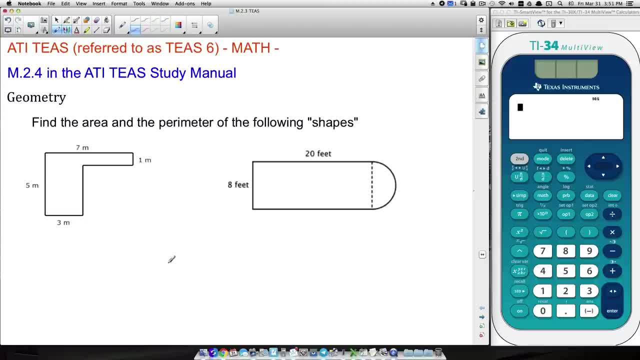 here. So let's go ahead and get started. We want to find the area and the perimeter of the following shapes. Something about area and perimeter is important, If you're following along in the ATIT area, to go ahead and mention area is always going to be in square units, square units And 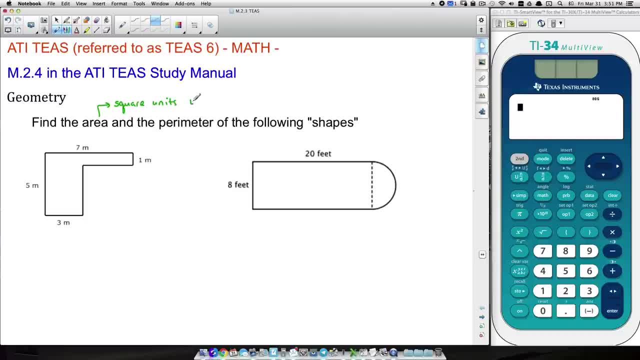 I'll show you why, but I just want to go ahead and stress that to you. Typically, we write that as unit squared, whether it be feet squared, meters squared, yards squared. Think about it: when you go buy a house or if you want to go rent an apartment, you want to know how big it is. 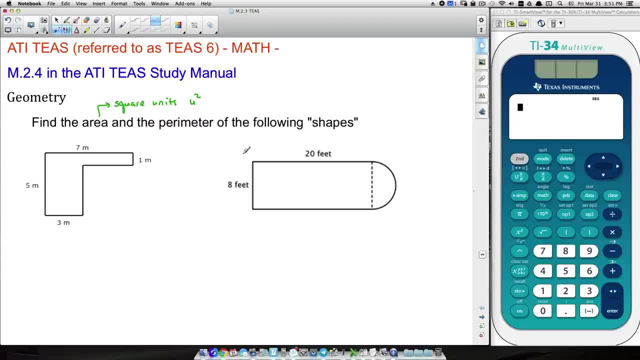 and typically that's the floor space and that's always given in like square feet or something like that, right, And then perimeter, that's just given in plain old units. So units, What do I mean by that? If you want to find, if you want to put a fence around your yard. 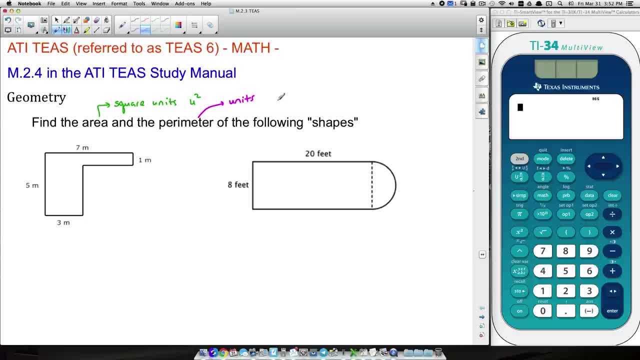 you don't want to know how many square feet of yard you have. You want to know the distance around your yard. so you just add up all the feet around the edge of your yard. That's what perimeter is the distance around a shape. So, given that, taking that into consideration, Now 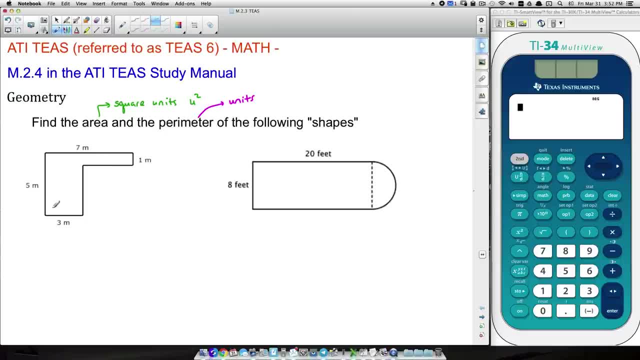 finding the area, the formulas, and if we look at this crazy shape right here, these are the ones that these are not identical to what you see in your ATIT study manual, but they're very similar. So if we want to find the area, we want to know how many square feet of yard you have, And if we 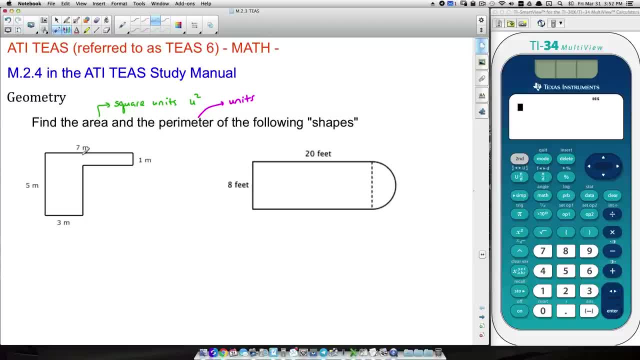 look at the area of this thing. well, it's a weird looking shape, but notice, if I cut it right here, if I cut it right there, really, what we have here are two different shapes. We have the area of the rectangle- okay, see that- And then we have another rectangle right over here. So we want to 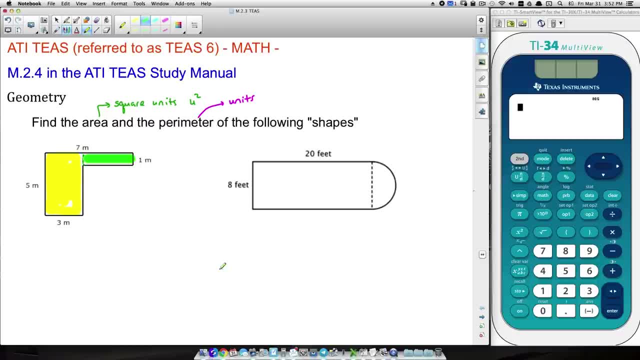 find really the area of two different rectangles and then we want to add them together. Well, it's still tricky. The area of a rectangle- there's nothing wrong with finding that, or there's nothing too crazy about that one. You probably are familiar with the area of a rectangle. We take the length. 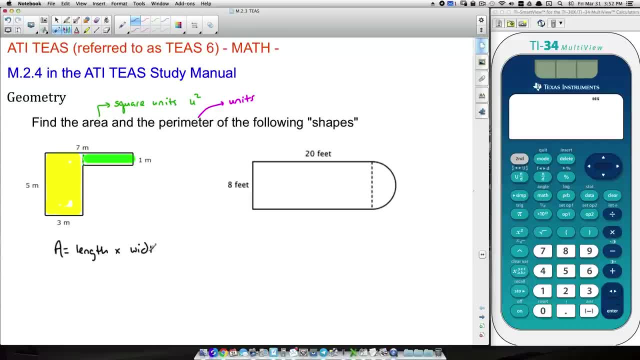 and we multiply it by the width. Some people refer to this as base times height, however you want to call it. Let's look at the yellow one. So the area of the yellow rectangle. I'm just going to highlight this A in yellow and that is not yellow, but now we do have yellow. 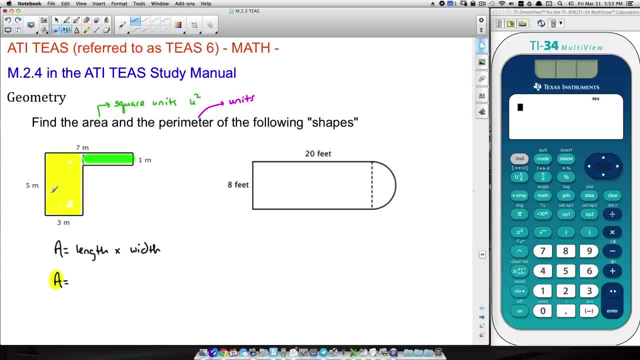 Let's find the area of this yellow rectangle. So we're talking about a length and a width. Well, notice this yellow rectangle. we have both of those measurements given to us. So the length: it don't matter which one you call the length, as long as you call one of them, the length. and 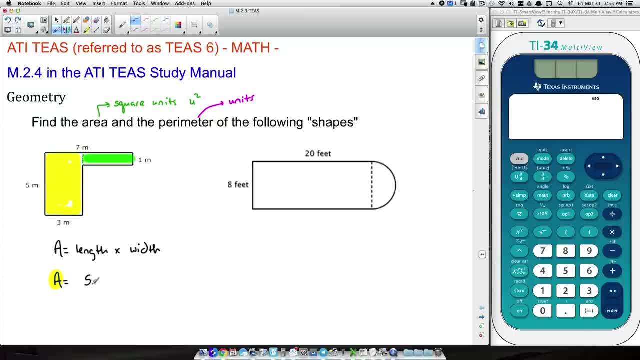 one of them the width. So how about five? It can be our length five meters and then our width can be three meters. Multiplying those two numbers together, we get 15, but it's not just 15, it's actually 15 square meters, or 15 meters. 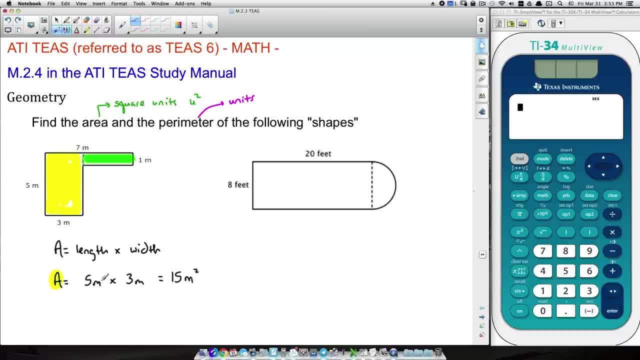 squared. And the reason why, if you're familiar with algebra, you almost want to think about it like you're multiplying variables. M times M is M squared. That's where we get those square units from. Now, that is only the area of this yellow piece. We have to come back and find the area of. 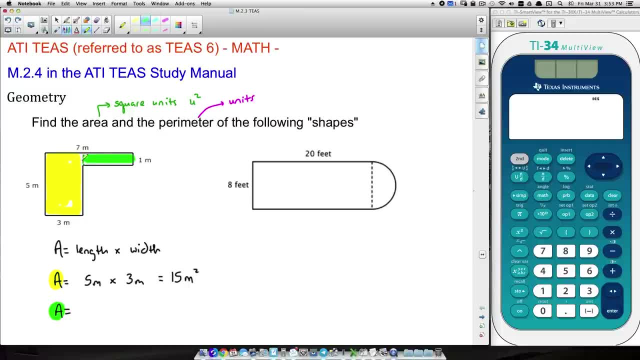 this yellow piece because we have two pieces that make up this. Think of this as like a living room in like a hallway or something like that, and you want to put carpet in it. All right, so if you want to lay carpet, you need like square meters or square feet or whatever. when you go shopping for. 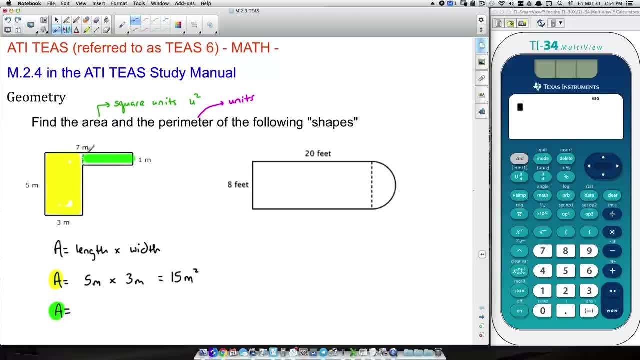 it. Now, we want to be careful with this here, and the reason why is because you may say, well, we got seven by one, and that is not correct. Sure, that says seven, but seven is actually the measurement all the way across this thing. And if I'm looking at just the green, all I really want is this: 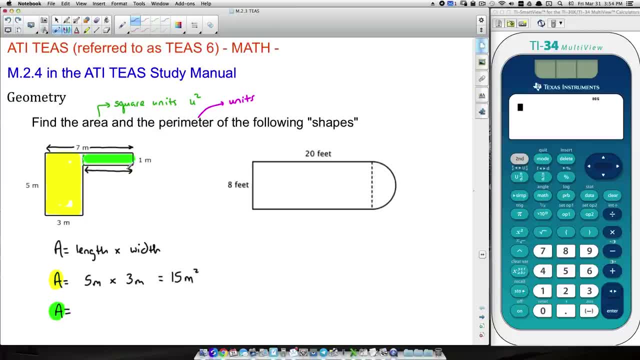 length. If we want to call this our length and call this our width, Again, it doesn't matter which one you call which. So the length and the width. How do we find this? Well, what do we know about this measurement from here to here? What do we know about this right here? From here to here. 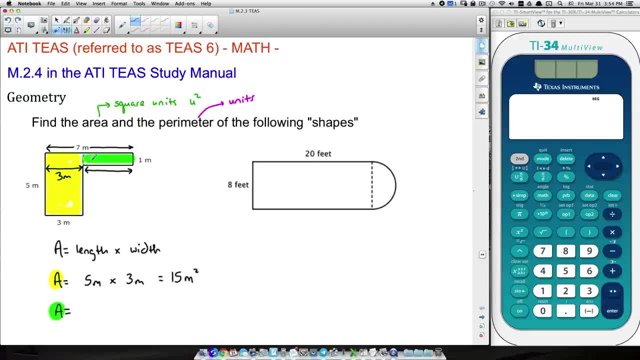 that's three meters. It's the same thing as this down here. So that's three meters, right there. Now let's take that into consideration. This is going to be four meters, because the distance from here to here is seven, right? And then we just take seven minus three. It tells us what we have. 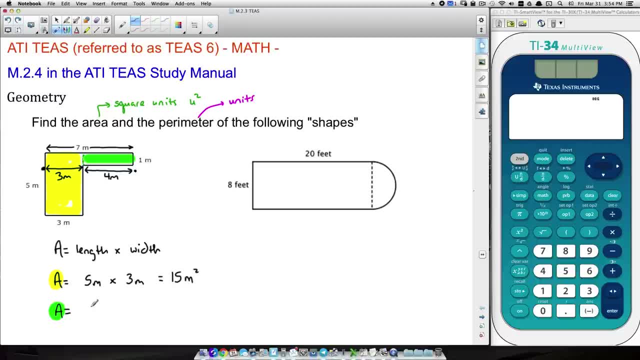 left over. So that's how we find the missing piece for this rectangle. So let's take our length of four meters times our width of one meter. Again, it does not matter which one you call which, And if we multiply those we get four meters squared. Our total area is going to be: 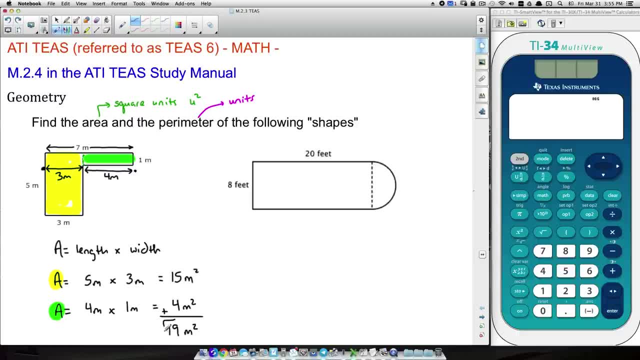 the sum, So we have 19 square meters. Now it goes to mention- I will not show it here, but I do challenge you to do this- You could definitely, definitely, definitely take this same exact shape that we just worked out and you could break it up differently. 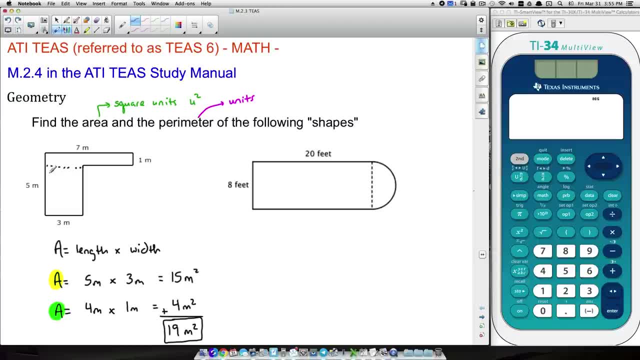 Break it up along this line right here, and you could find the area of this rectangle and you could find the area of that rectangle. You will get the same answer, but your two regions, these two numbers here will differ, but still the sum of those will be 19 square meters. 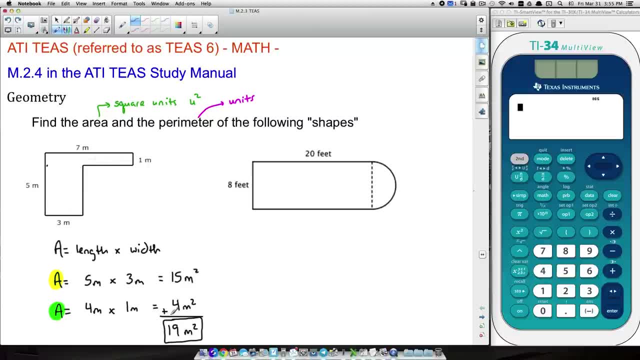 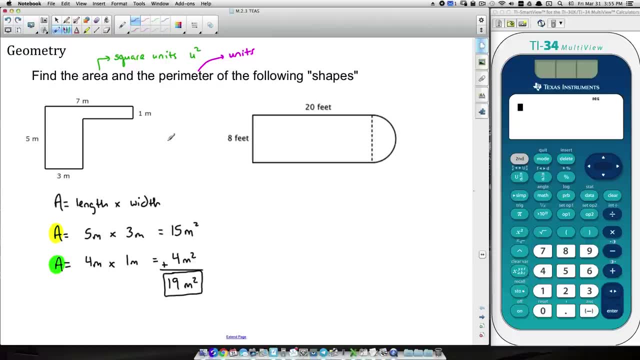 I challenge you to try that. If you have any questions, leave a comment in the comment section below. Now let's find the perimeter of this shape as well, because we've got to find both the area and the perimeter. Well, I did erase some things, but I want to keep the four meters. 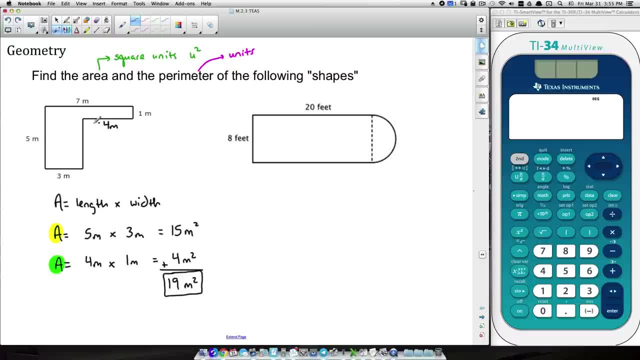 here. That's very helpful right there, because the four meters is the distance from here to here. It's the length of this section right there, And the reason why I want to keep using that is because the perimeter is going to be the distance around this shape. So we're talking about like the wall. 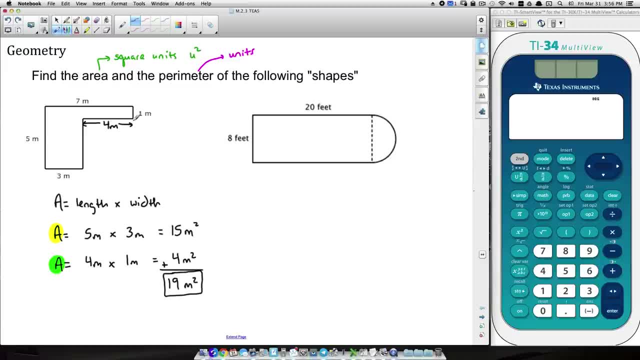 of this living room, in this hallway. You know what's the length of all these walls, so to speak. Now we're still missing one more piece as well here, because we need to find the distance from here down to here as well before we can add up the four meters. So we're going to keep using that. 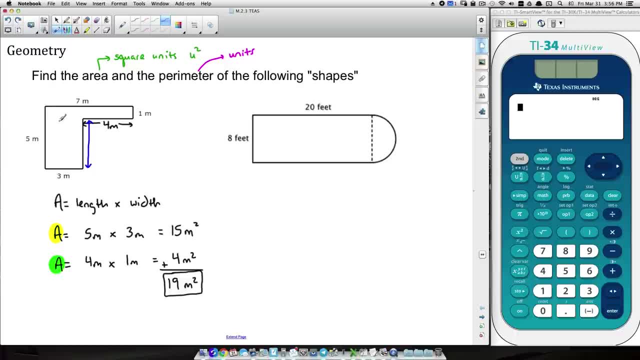 up all these sides. Well, we can take a very similar approach to what we did while ago with this piece, Since we know that the distance or the length from here all the way down to here is five, that means that the distance from here down to here also has to be five, right Well? 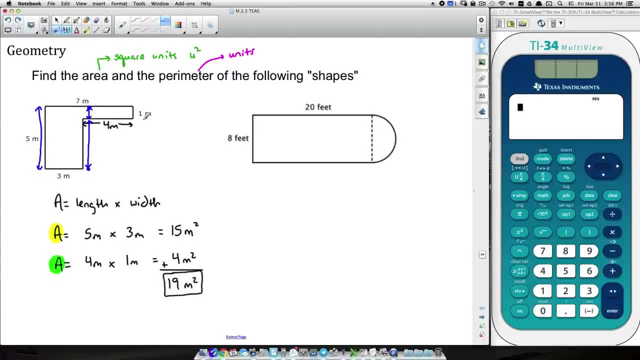 what do we know about this? What's that distance right there? What's that length right there? That length is one. So if that's one meter from here to here, then we've got to have four more to give us that total of five right there. 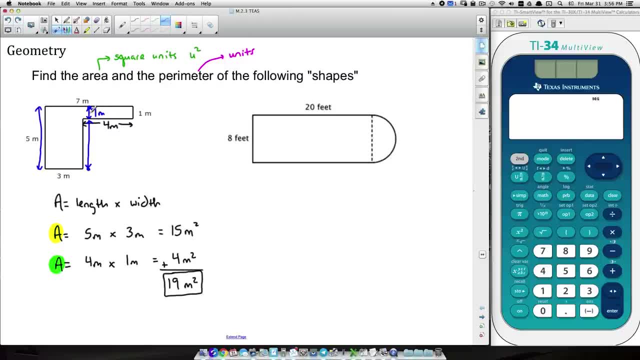 All I'm doing is taking the total length, five, and I'm taking away that one because I don't want to factor that into this piece that I'm trying to find here. So that has to be four meters. Well, lucky for us. I mean, these ended up being the same numbers And it turns out we just add up. 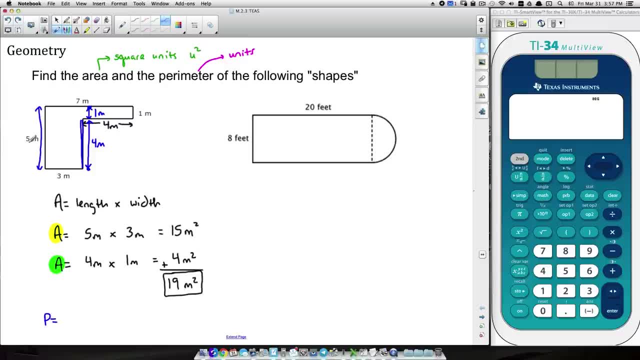 all of these sides, So the perimeter, adding them up. I'm going to start with the five here and I'm going to go counterclockwise. So five meters plus three meters, plus four meters, plus another four meters. right there, I'm just adding up the sides on. 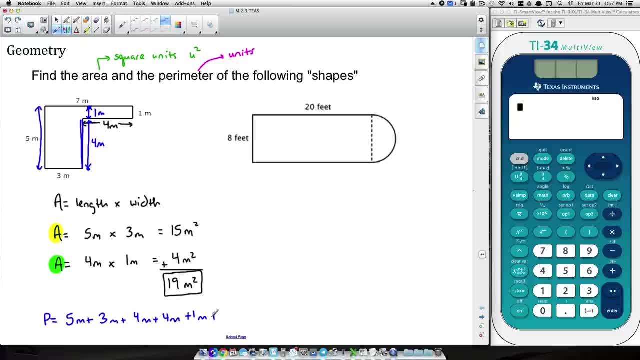 the outside, and then plus this one meter, And then, last but not least, plus the seven meters. So if we add all these up, five plus three is eight. Eight more gives us 16.. That's 17.. And then that's going to be what? 24.. So 24 meters right there, That's going to be the distance. 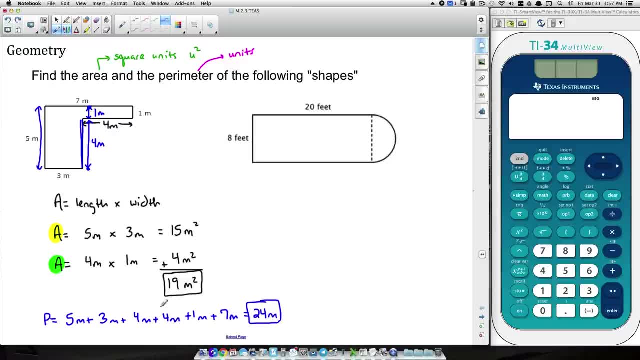 around this thing And notice: I said meters, I didn't say meters squared, because we are combining like terms, so to speak. Think algebra: In the algebra class, when you combine like terms, we just add up all these coefficients, add up all these numbers. 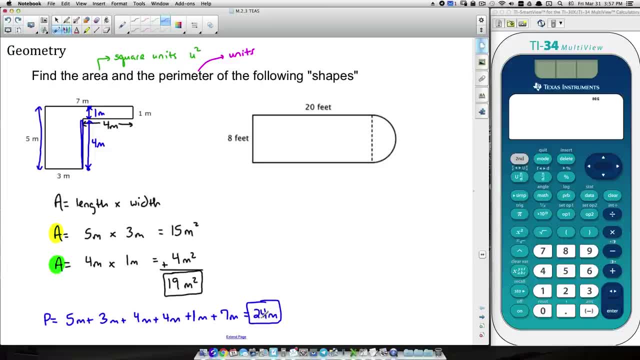 That we have here And then we write that variable down. We're really that's what we're doing when we find perimeter. I hope that makes sense. Now some other things to point out in this particular example. you know this is going to be a little weird, but I want to explain it. 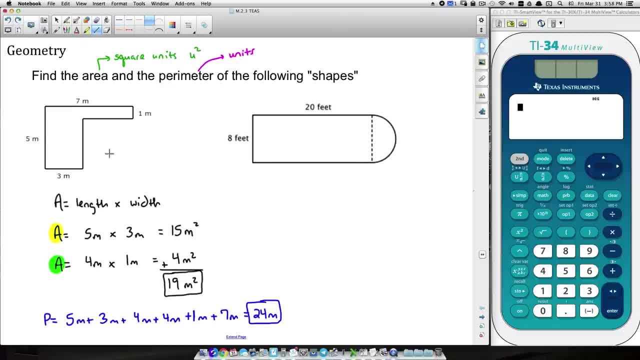 anyway, When you have what looks like a rectangle with like a single section missing, like this off of a corner, I don't really like I don't teach it this way, But if you notice this like this is going to be the same thing as that distance right there And then this distance here or that. 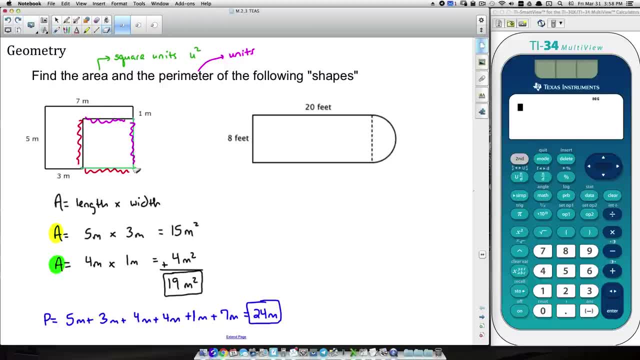 link there is going to be the same as that link there. So you know, let's look at that red and that pink. They're going. the pink is going to be the same as that one. The red is going to be the. 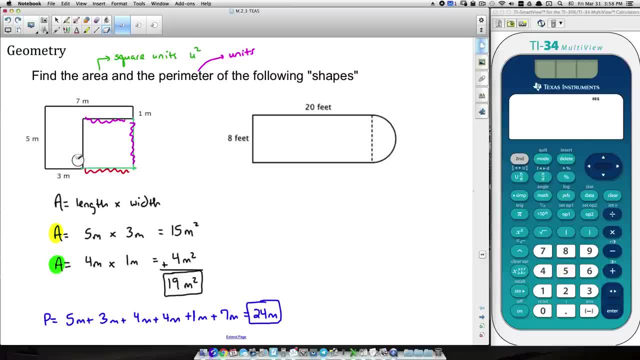 same as that one. Now we are making some assumptions here. We're making assumptions that all of these angles that we have in here are right angles, And we're going to make that assumption. You should pretty much just be dealing with right angles with these types of shapes on. 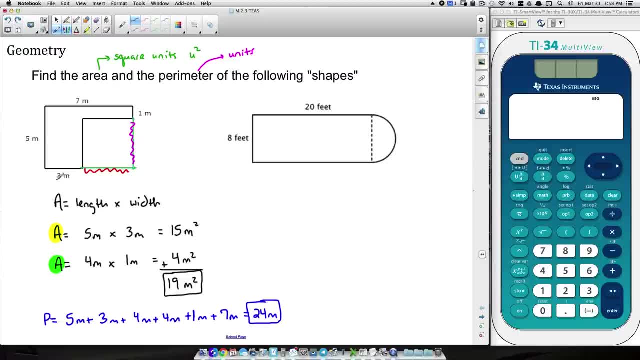 the tease test. Well, with that said, we can just totally bonk out this three right here, because we, we know the distance across this whole thing, don't we? The distance across this whole thing from here to here is going to be the same thing. 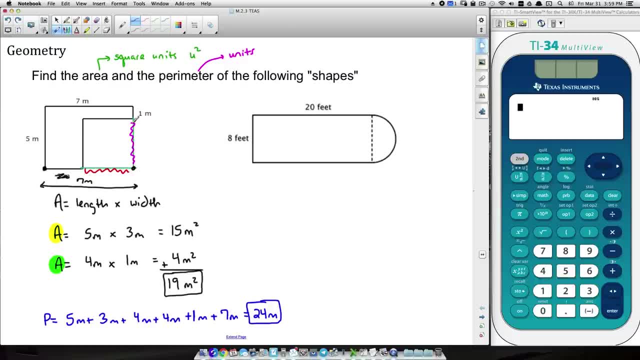 as that up there. So that's seven meters just taking a different approach here, And the same thing will apply over here to this side. We can just throw away that one because we know the distance from here to here, the distance along that line right there, that whole line from here. 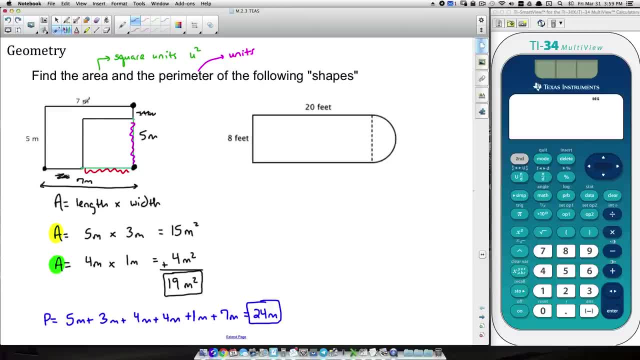 to here is going to be five meters. Well notice, if we add this up, I'm five plus seven. Now, really, that's a crazy shape now. So it's going all the way around: Five plus seven is 12.. And then we got. 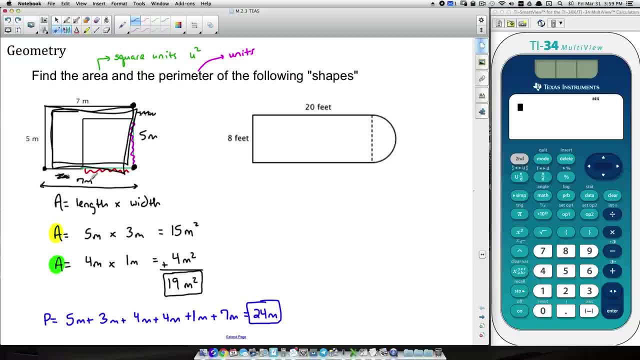 12 more because we got another five and another seven. So 12 plus 12 gives you the 24 square meters. Just a little trick right there, I don't. I mean, I wanted to mention it to you because you may hear somebody else mention that It's hard for me to cover every single thing you're going. 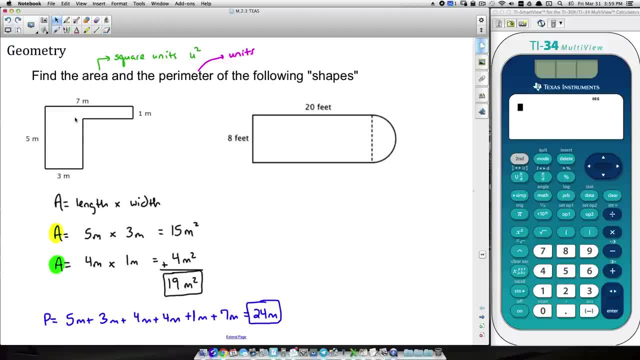 to run across, but just just a little little fun fact. All right, So that's the two answers for our first problem. Now the second problem here: what do we have going on in this problem? That's why I over here, because we're going to round this thing off to find the perimeter of this thing. Now. 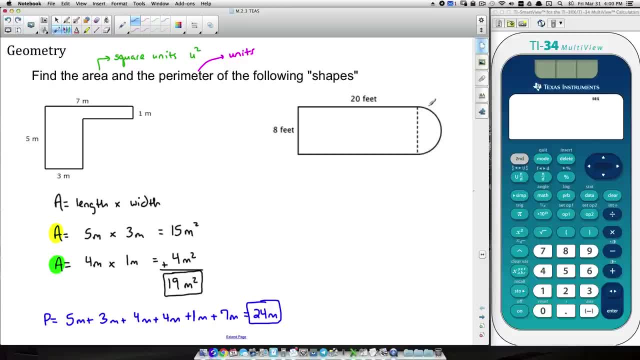 what we have here is like a rectangle, And then we had this half circle and we can make the assumption that this is a half circle because you you have one pretty similar to this in your ATIT study manual. but we're going to find the area and the perimeter of this thing. Let's start off. 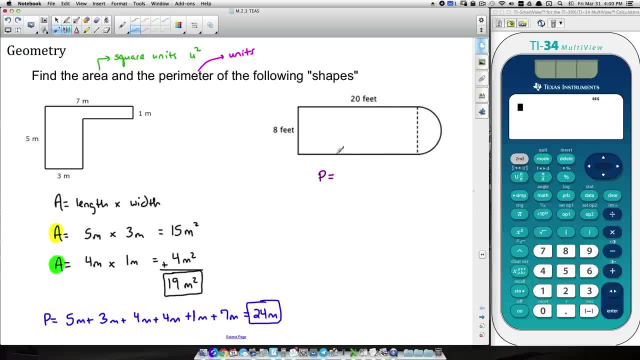 with perimeter first this time. Why not? So perimeter is equal to well, we got that 20,. we got eight and we got 20, but notice, I stopped there. So we got 20 plus eight plus 20.. So 20 feet plus eight feet plus 20 feet. Now we do not, you do not count this, We don't want to cut. 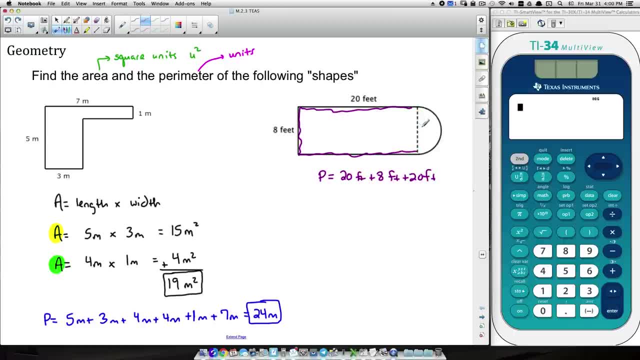 across the shape to find the perimeter. So we do not count that dotted line. That dotted line is pointless to me. but to be quite honest with you for right now, well, what are we going to add on? We want to add on this distance right here, Okay, And now you know. okay, well, what is that? That's. 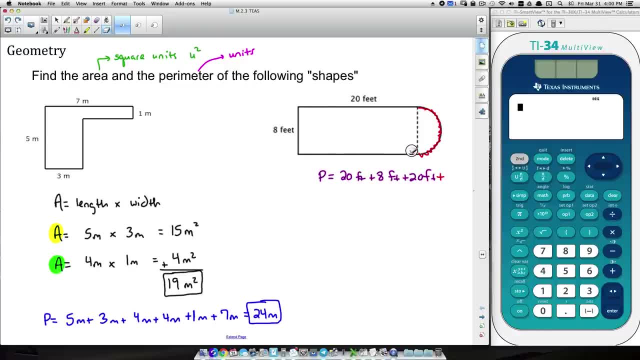 a circle, right? Uh yeah, Kind of sort of, but it's a half circle. It's a half circle, And when we talk about perimeters of circles, um, what we really want to talk about here is the circumference of a circle. 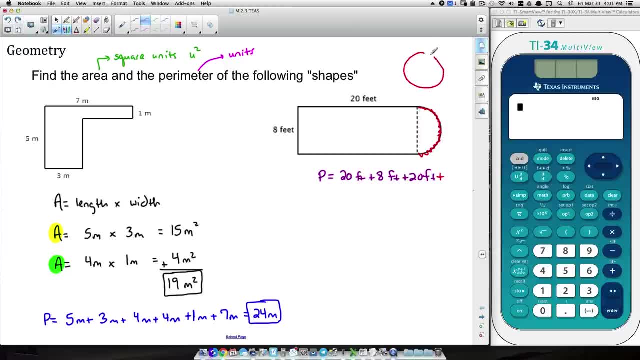 but the circumference of a circle covers the distance all the way around. So if I start right here on this dot and I go all the way around this ugly circle that I've drawn here, um, that would be the circumference of the circle. Well, I'm not going around a whole circle, I'm going a half. 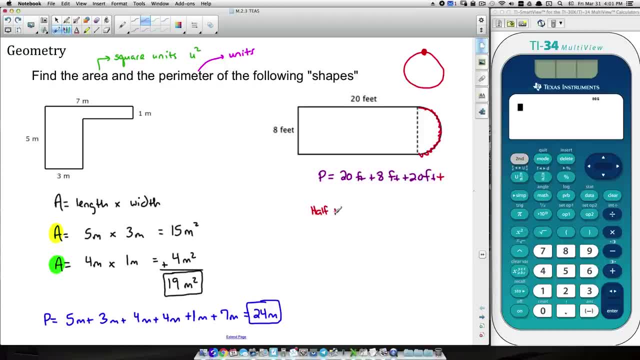 circle. So what we want to find here is half the circumference. Now, this is a formula, So you got two formulas for circumference. Um, I have a video on my channel as well that covers a lot about circles, where I discuss formulas and where the formulas come. 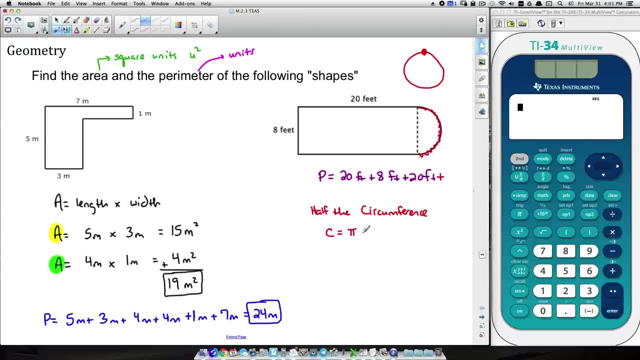 from. So I encourage you to check those out. but the two formulas for the circumference of a circle are going to be pi times D, or you can use circumference equals two times pi times R. D is the diameter, R is the radius. Now, assuming if you're somewhat familiar with circles, maybe you 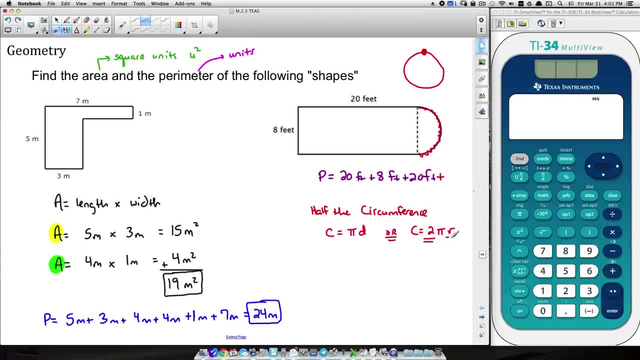 're not. it's okay, But if we take two times a radius, two times a radius is going to be this diameter. That's why these two formulas that you see here are the same. Now, which formula do we want to use? It doesn't really matter. Well, okay, well, what's going on? Okay, We got to have a. 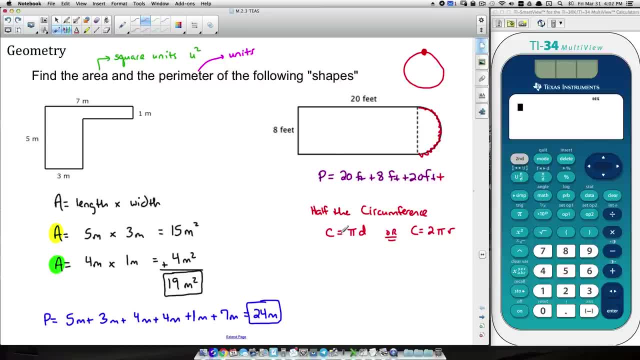 diameter. We got to have a radius to find the circumference. Well, um, to do that, uh, this eight feet, is this length here, That length right, there is also eight feet. So from here to here, that is the diameter of that circle, the diameter of that half circle. So let's use this formula: 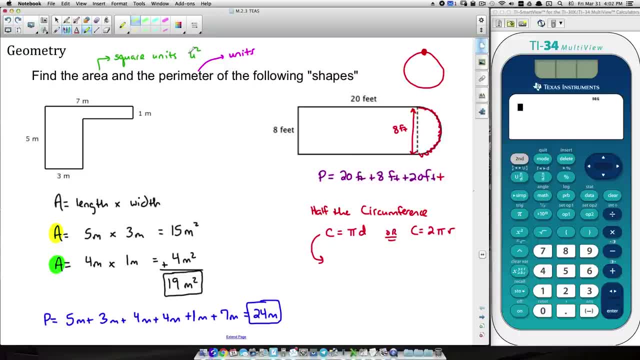 right here, but bear in mind I am, I haven't, uh, I said it, but we're not talking about it just yet mathematically. but we got to find half the circumference. So, um, circumference of a circle. 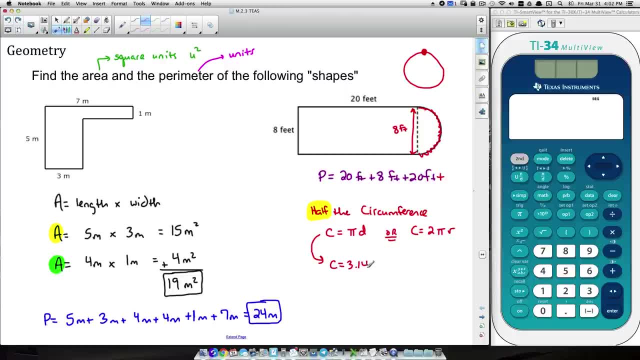 is pi D, So circumference equals and I'm just going to use 3.14 because your calculator does not have a pi key on it on the ATITs test. So 3.14 is what we commonly use for pi. And then we 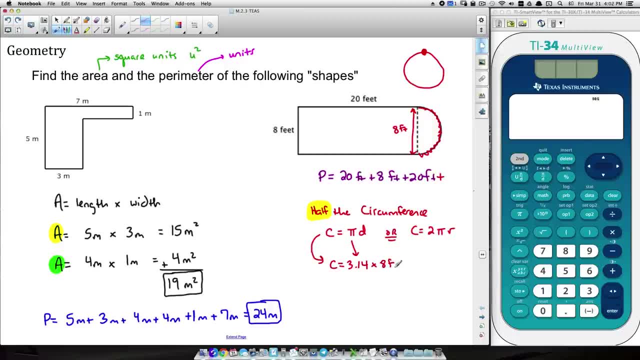 multiply it by the diameter, which is that eight feet. Well, let's just come over to the calculator: 3.14.. Let's multiply by eight and we get 25.12.. So, uh, this is approximately 25.12 feet. Now, what we want to be careful here is this: Notice I said. 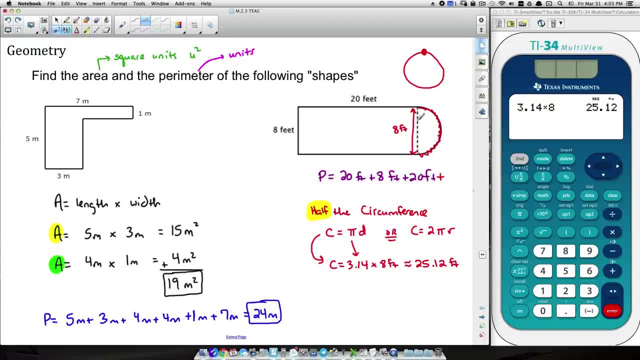 half the circumference. This would be the distance around the whole circle, Had we had a whole circle up here, which we don't. So what we want to do to this thing is: we want to take half of it. We want to take half of it, We just divide it by two. So we're going to take this circumference. 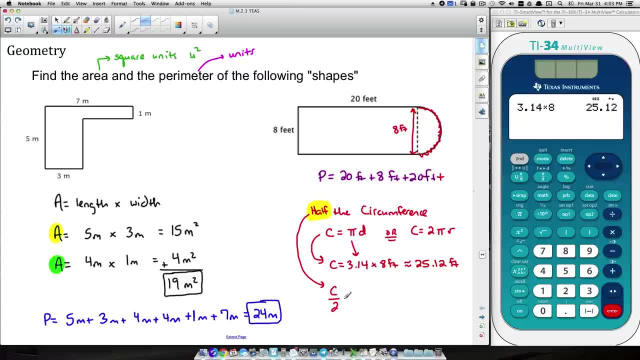 we have right here circumference and divide by two. Therefore, we're taking that 25.12 feet and we're cutting it in half, dividing it by two. So divide by two, That's going to take the 25.12, divided by two, So we get 12.56 feet, 12.56 feet. So this piece here is the missing piece that we. 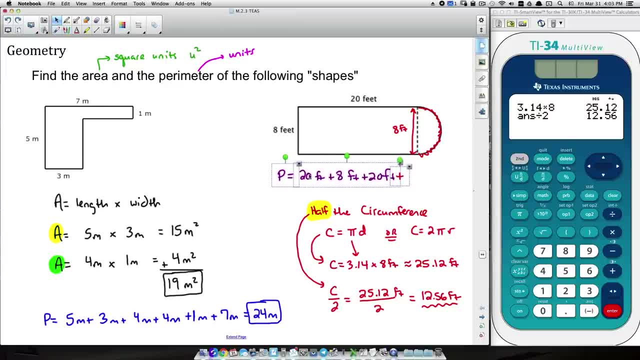 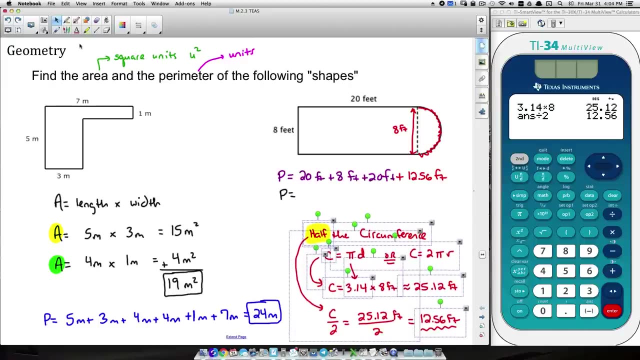 need to add up in here into our problem. So I'm going to take that on. So we get 12.56 feet and now the perimeter when we add up all these sides. let me slide some of my stuff out of the way here. so, just adding it all up, they're all in feet and we're not. we don't have to convert. 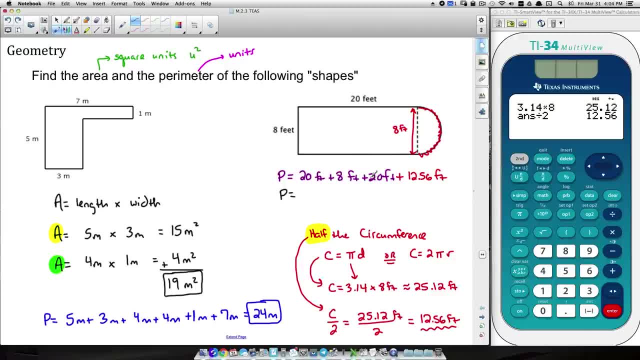 anything. so 20 plus 20 plus 8, that's gonna be 48. so 48 plus 12.56 that's gonna be 50.56- or, excuse me, not 50 but 60.56. so that's going to be the perimeter of our weird looking shape here: 60.56. 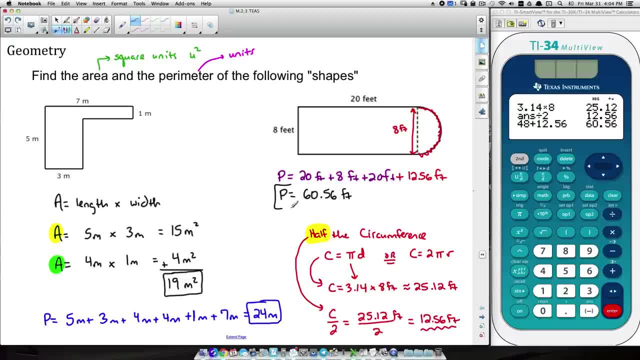 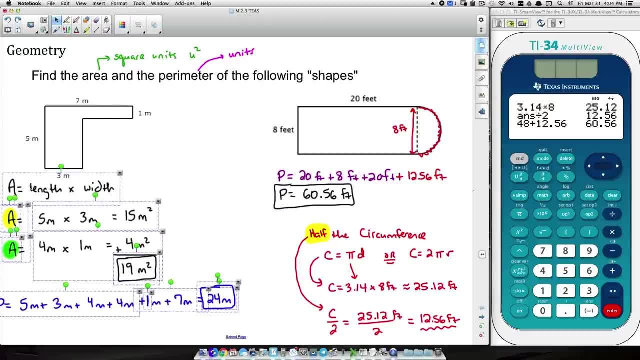 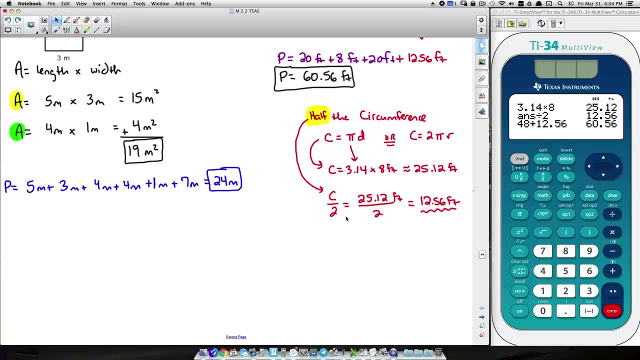 feet. okay, that's the perimeter. now let's find the area. so let me do some cleaning up here. of course I could erase everything, but I like to save these files for future reference. so I'm just gonna tell you what. we'll go down a little bit and we're gonna take 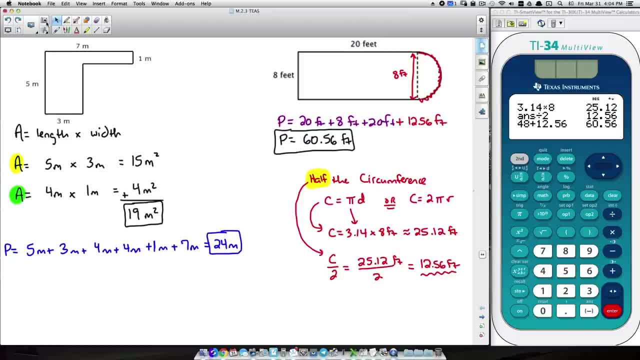 let's see, we should be good right there. okay, so the area: what in the world do we have going on here with the area, the area of this shape? well, if we break it up into two pieces, kind of like what I did over here, I broke it up into. 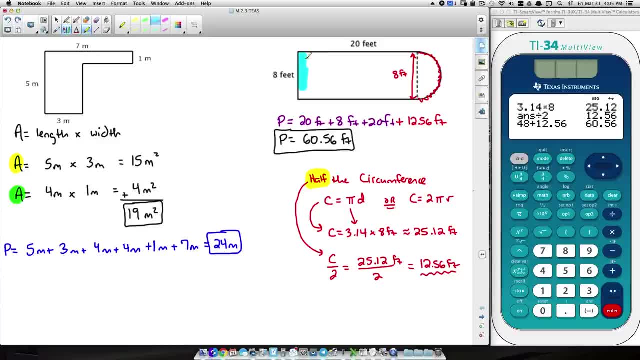 two rectangles. we can't break it up both of both of these sections up into rectangles, but at least we can look at this blue piece here which is a rectangle, and then we can also come and look at this pink section right here which is a half a circle, which I've already mentioned. but now we 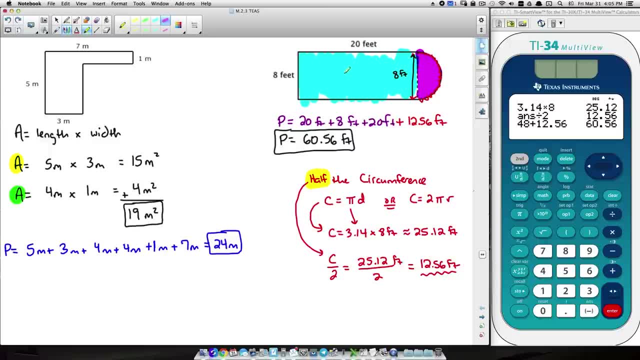 don't want to talk about circumference anymore. so we want to find the area of the blue region and the area of the pink region and very similar to what we did over here. we want to add them up. add them up, okay. so the area of our shape. I'm gonna get this stuff out of the way. that goes with this. 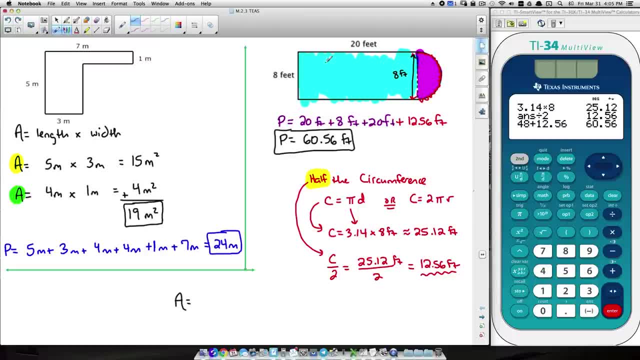 over here, but the area of this shape right here we want to take the area of our rectangle, where the area of our rectangle is going to be 8 feet times 20 feet, very similar to what we did back over here when we found the area of our 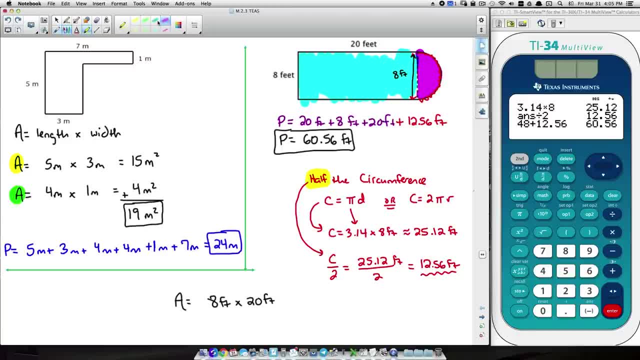 rectangles, and this is going to be just the blue region. okay, so we have what? 168 times 20 is 160, and remember feet times feet. we're finding area. so we have square feet, square units, don't forget that. and now let's come and find the area of our dark pink. 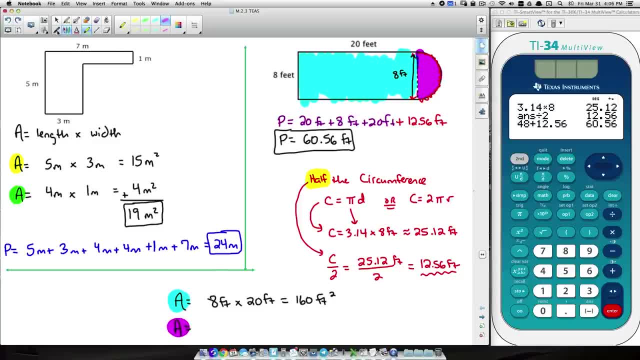 region, which is the area of a half a circle. well, the area of a circle is there's only one formula that you need to know, that you need to memorize, and that is PI R squared. PI R squared. now, this is the area, this is the formula for the area of a whole circle. so what we want to do is we want to 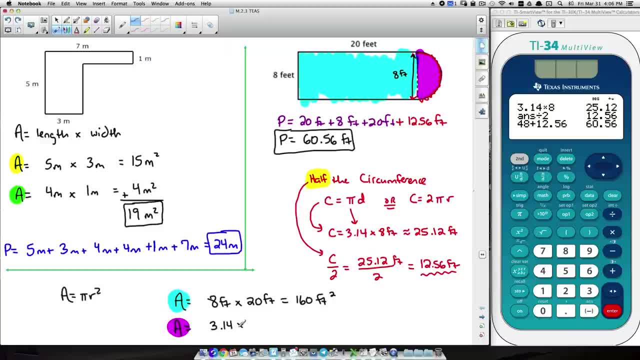 do is we want to take PI times now our radius up here. I did use the diameter because that is what that is. the the radius is always going to be half the diameter. the radius is really going to be the length of the line that goes from here right to our edge, and that's half of the distance all the way across this. 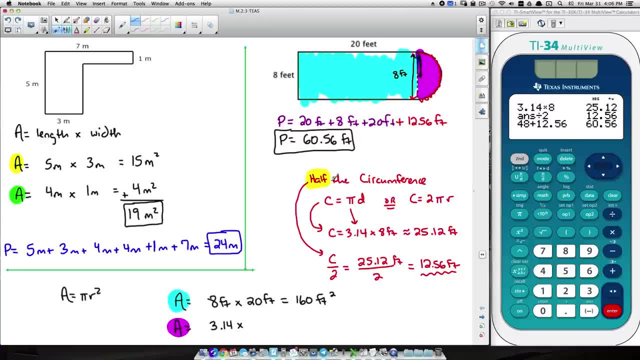 circle right here, this half circle, so half of that is going to be 4, so our radius is going to be 4 feet and we want to make sure we square that. and but now notice this Formula: PI times radius squared. PI times radius squared. well, what we 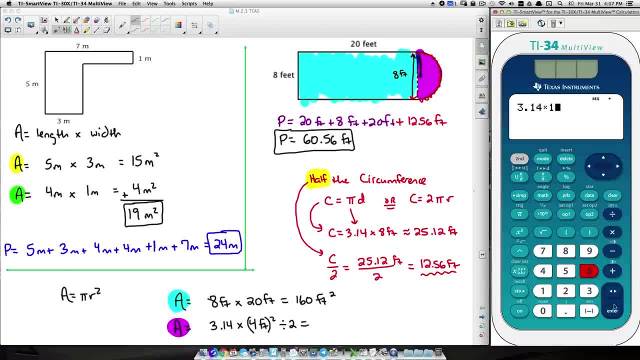 4, so 3.14 times 16. that's the area. if this thing was a whole circle, roughly 50.24 square feet. notice square feet, notice feet, times feet or feet squared right there. but we want to divide this by two, so divide by two, press enter and we got 25.12. ironically, this is crazy: 25.12 square feet. 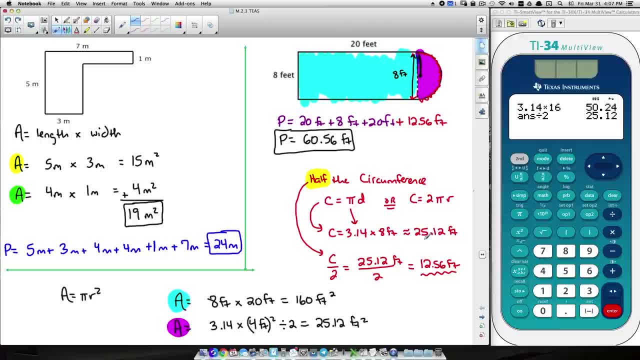 what did i laugh about it? we're getting that number there. do not make that assumption. that's just coincidental plus. you know, we ended up dividing that by two anyway. circumference and area: there's two different formulas. there's two different ways of finding them. don't think there's. 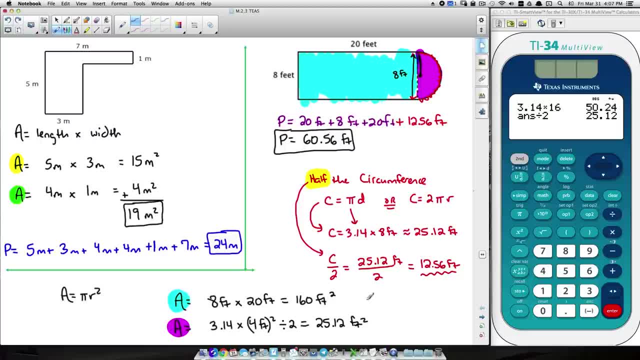 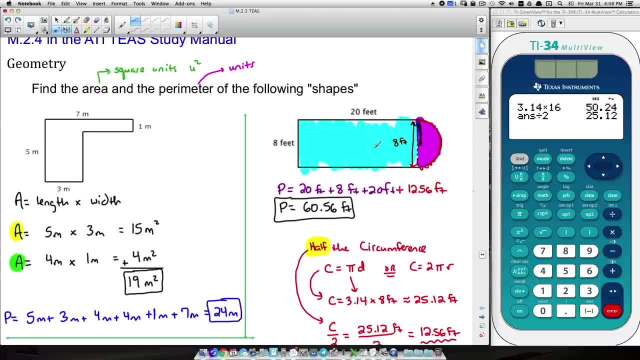 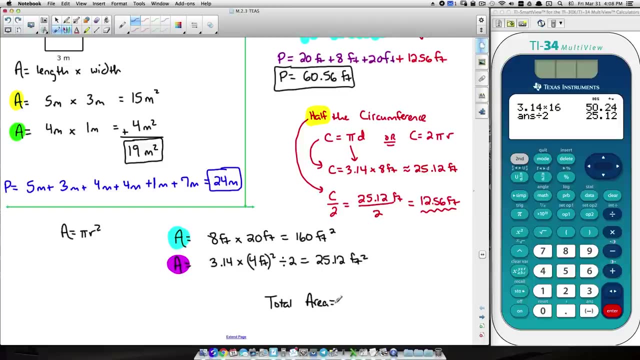 ever going to be a real strong relationship like that that you're always going to get the same number somehow? no, that's not the case. so with all that said, uh, let's see here. okay, what's the total area. we got to take the blue plus the dark pink. we got to add those together, so total area is going: 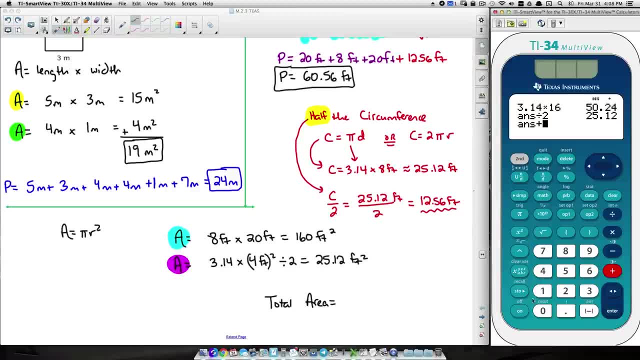 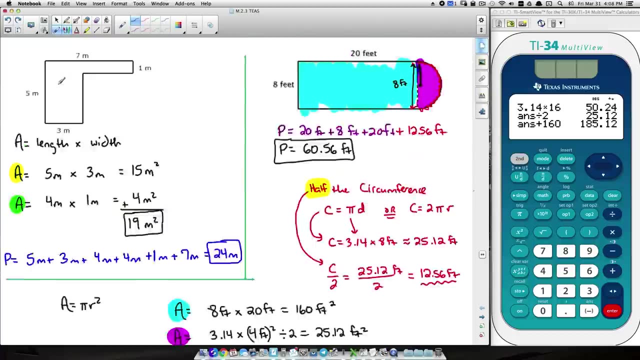 to be the sum of these two. so let's take that 25.12 and let's add the 160 to it, so that's going to be the what: 185. yeah, so 185 point 12, 185 point 12 square feet. all right, so that's a lot. now i want to cover some word. 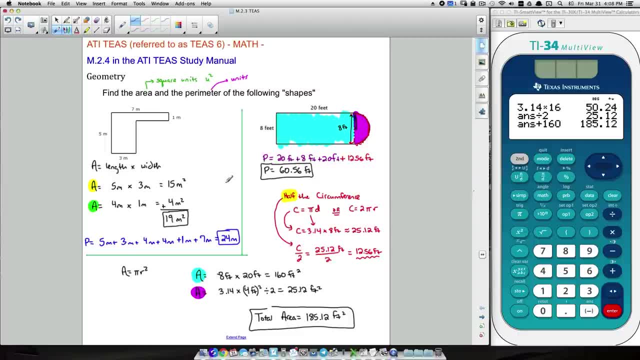 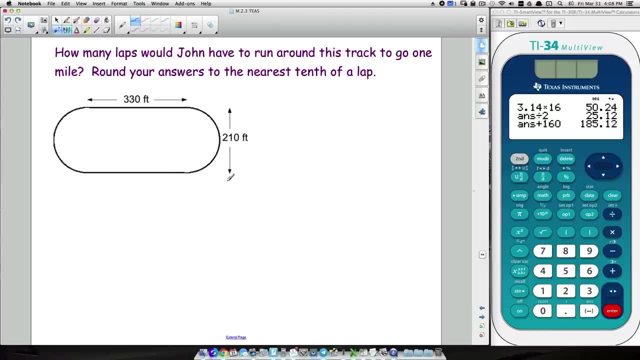 problems with you because the the t's test might not necessarily say, hey, find the area, find the perimeter. so we're going to look at two examples where it does not say find the perimeter or find the area. you need to know what to do. and then, plus, you got to read the problem a little bit. 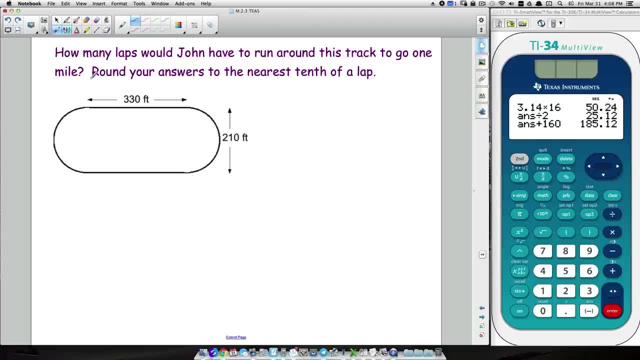 more carefully. so these last two are going to be a little bit challenging. um, how many laps would john have to run around this track to go one mile round? your answers to the nearest tenth of a lap. okay, so let's just say the starting line is right here. okay, this is the starting line start. okay, so he's going to run one lap, boom. 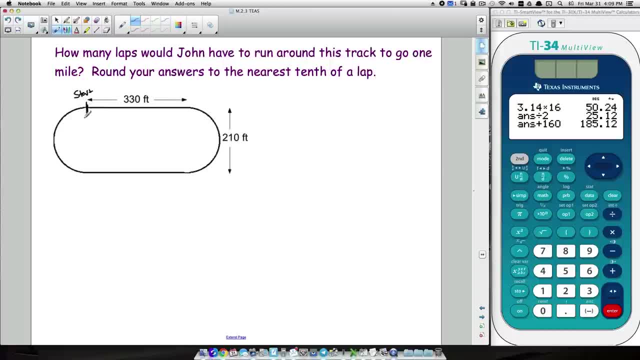 boom, when he goes like that, when he goes back to the start, that's one lap. well, what we want to figure out first is is: well, how long is one lap? how? how long is one lap? well, that is going to be the perimeter of this shape, right? well, good news, we got some easy parts this straight away here. 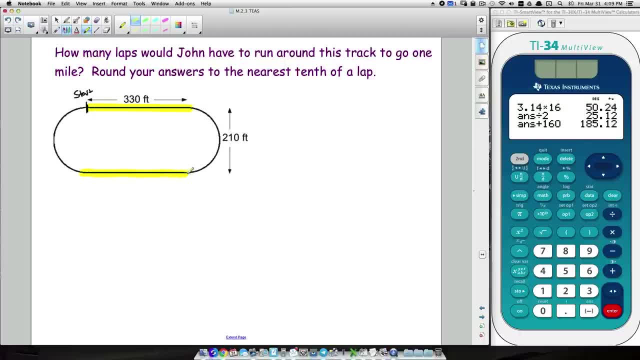 330 feet, this straight away here. 330 feet. well, what about this? oh, here goes that half circumference again. right, we got a half circle. oh, look over here, here's another half circle. hello, think about this now. this 210 does not correspond to the length of this curve. the 210 corresponds kind of like the. 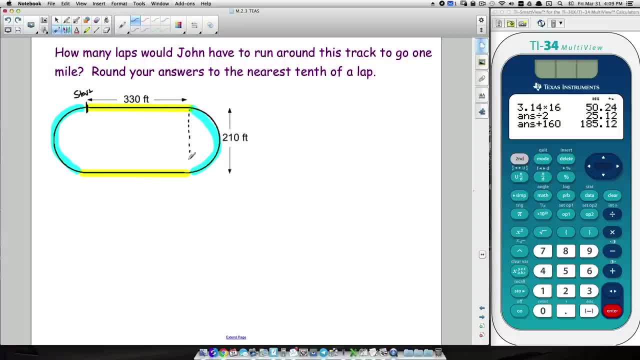 way we had, or, like you know, the dotted line. it goes across here. so this right here, the diameter, if you will, will be 210 feet. well, so the distance, let's say one lap, one lap is equal to automatically. if he starts here, he's gonna have. 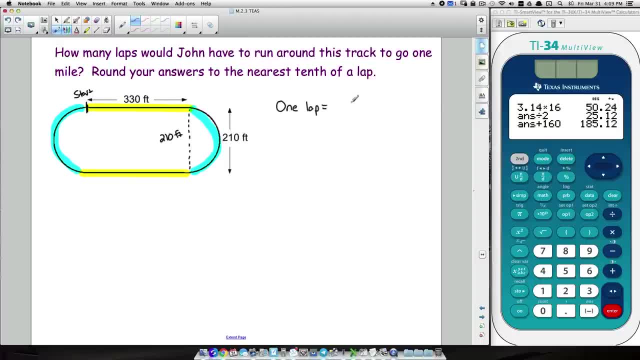 to run. eventually he's got to run this straight away and then he's got to run this straight away, so let's just go ahead and add those up, so 330 feet plus 330 feet. but then we got to count these two half circles. well, two half circles make a whole circle. think about that, this half a circle. 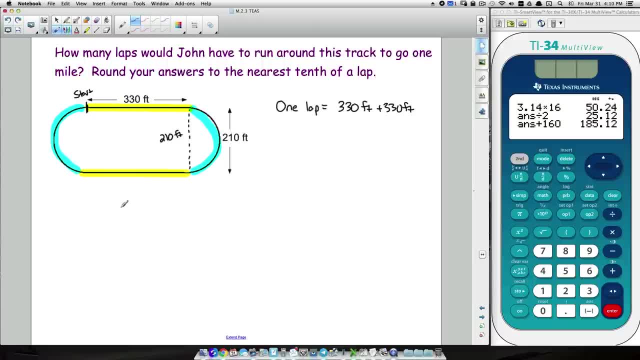 is gonna be half the distance. well, this is gonna be another half a distance. so, really, even though we have two sections that make up, you know we got a half circle here and a half circle here- honestly you can think about it as being a whole circle. with that said, let's use the circumference. 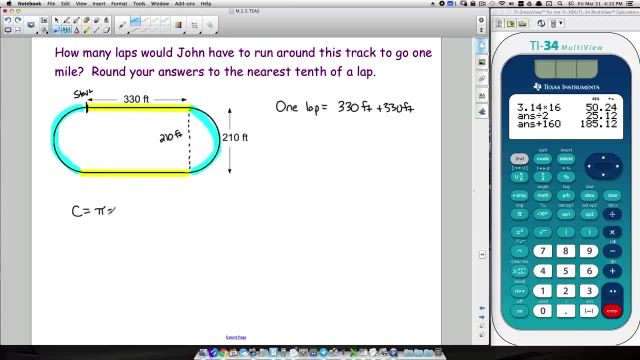 of a circle. we can either use two power or pi D. I'm going to use pi D. pi times the diameter. so therefore pi is three point one, four. our diameter is going to be 210 feet. that's the distance all the way across this half circle here. so 210 and that's gonna be feet. so three point one, four times. 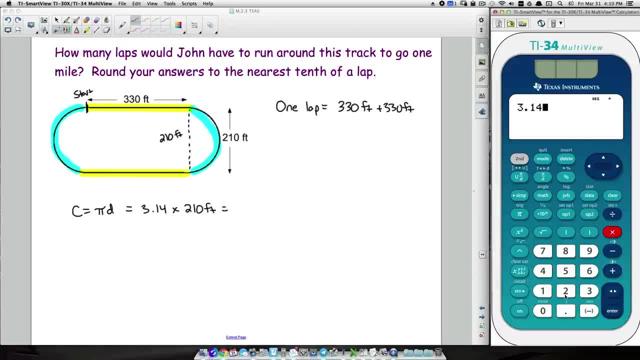 210. let's see what we get there: 3.14 times 210.. now again, I'm not going to divide by two here. and the reason why I'm not going to divide by two here: if it was just one half circle, then yes, I. 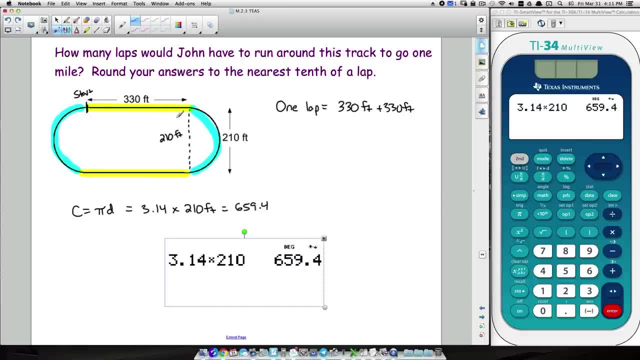 would divide by two. but since we have a half a circle here and a half a circle here, that makes a whole circle, so we can just use straight up the straight up formula for the circumference of a whole circle. so we want to add that on as well. plus six hundred and fifty nine, point four: 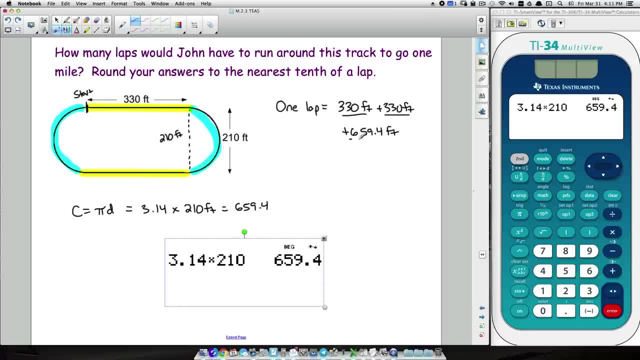 feet. so let's add up this measurement, this measurement and this measurement, and that's going to be the distance or the length of one lap. so one lap, one lap, is equal to take the 659.4 and we're going to add 330 plus 330. well, really that's the same thing as adding 660, so we get 1319.4 feet. 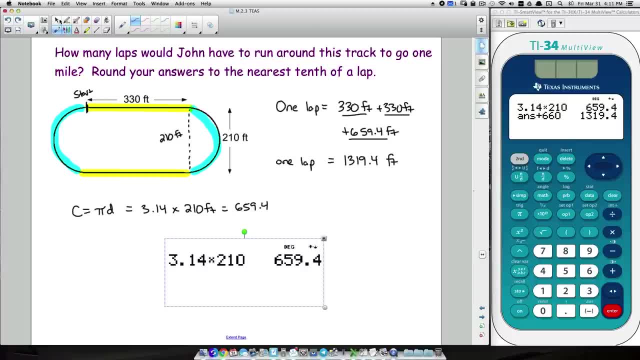 well, we're still not done with this problem because we have to read this question very carefully. how many laps will John have to run around this track to go one mile? this is in feet. you have to be careful when you read these problems. I didn't mention that yet because I was hoping maybe you saw that and 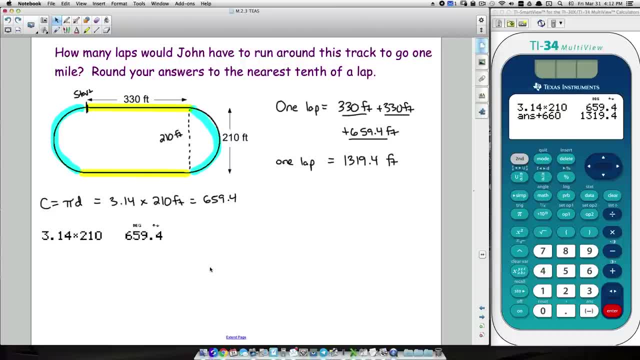 you were, you might have been thinking: hey, I wonder if he's going to mention that. here we go. well, this thing I wrote over here one lap. let's set up a proportion. one lap is 1319.4 feet or so, approximately that, and we're going to be okay with that. 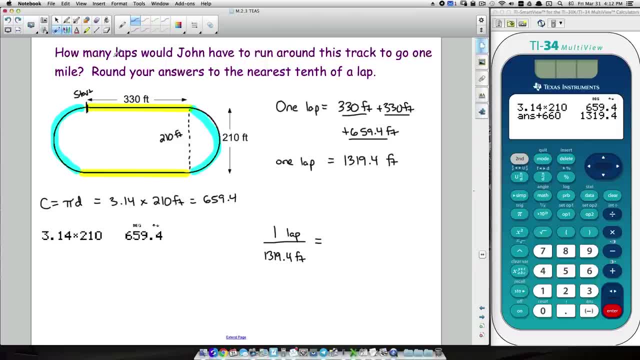 all right, well, equal to. we're trying to figure out how many laps. we don't know how many laps. well, since I have laps at the top here, I'm going to set up a proportion and say x slaps over. now what do we got to put down here? we have to put feet. well, I mean, I don't know because I've never taken the. 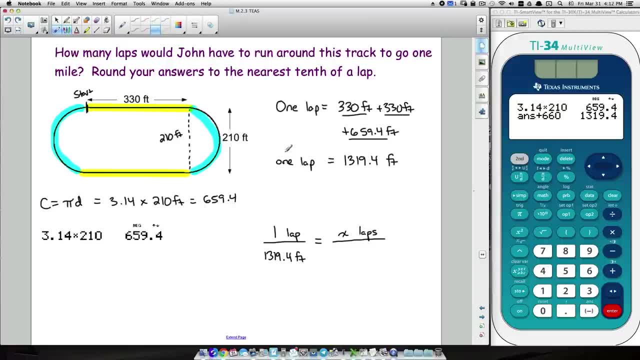 tease test I. I get feedback from students who take it from the classes that I teach for the tease test and they they do say you got to know some of your conversions, but then on some questions they'll give you the conversion. conversion here is: one mile is the same thing as 5,280 feet Basically, if you take a ruler. 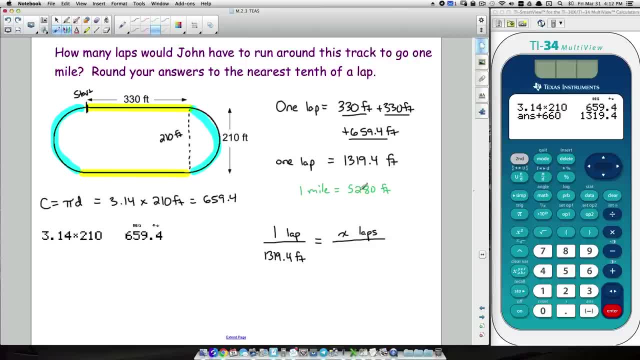 that's 12 inches long. take a ruler one foot long. if you line up 5,280 of them, that will be a mile, All right. So that's what we want to use. One lap is this many feet X laps. 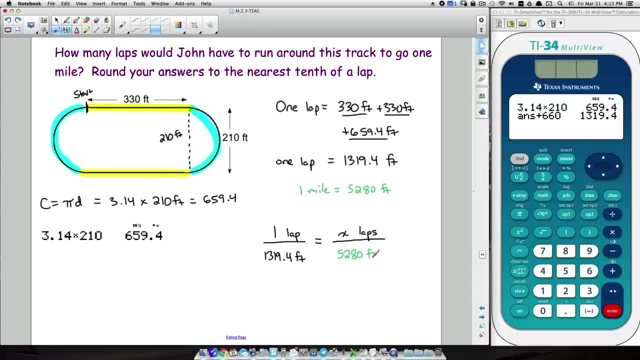 is going to represent 5,280 feet. That's going to be one mile Because, remember this right here is one mile. So if we can figure out X, we're going to figure out how many laps it will take to go one mile. What we can do here is we can cross, multiply and divide. 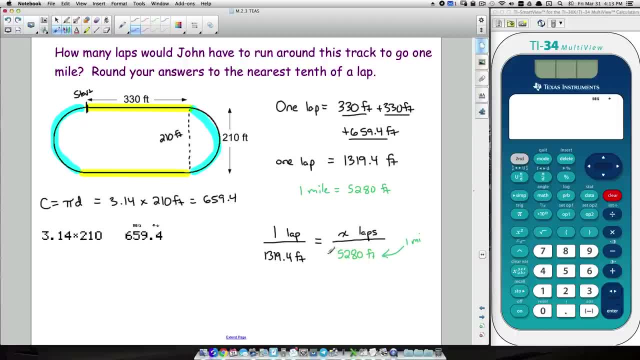 That's how we solve proportions. We've seen that in a video prior to this. So cross multiplying one times 5,280 is just 5,280.. And then we want to divide by the number that's getting multiplied by the X. That was the shortcut I gave you back when we looked at proportions. 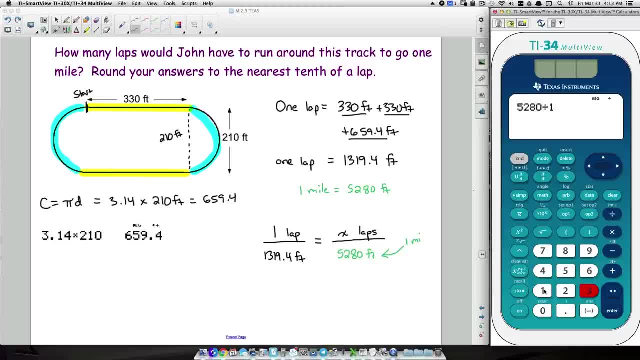 So we want to divide this by 1,319.5.. So we need to go roughly. okay, it says round to the nearest tenth of a lap. Well, pretty much, if he runs four laps, I mean just a hair over four laps, I mean not even a fraction. 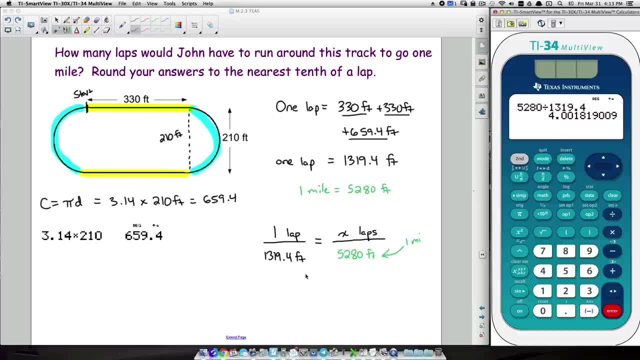 of a foot really. So four laps is what we're looking at. So X is equal to four laps And even if we need to round to the nearest tenth, as you can see that zero is going to tell that zero in the tenth spot to stay the same. So four laps. John would have to run four. 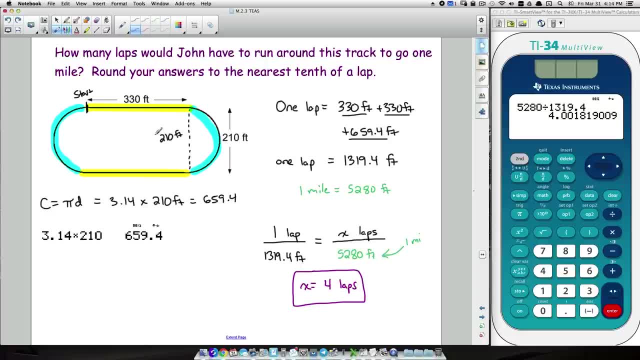 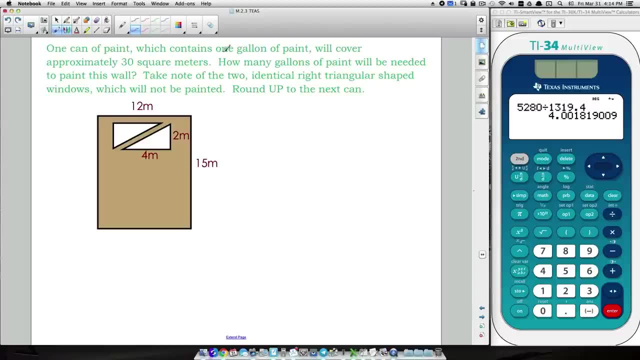 laps around this track to go one mile. I hope that makes sense. And now our last problem. So we got one can of paint which contains. one gallon of paint will cover approximately 30 square meters. How many gallons of paint will be needed to paint this wall? Okay, I'll tell you what: how many cans of paint. How? 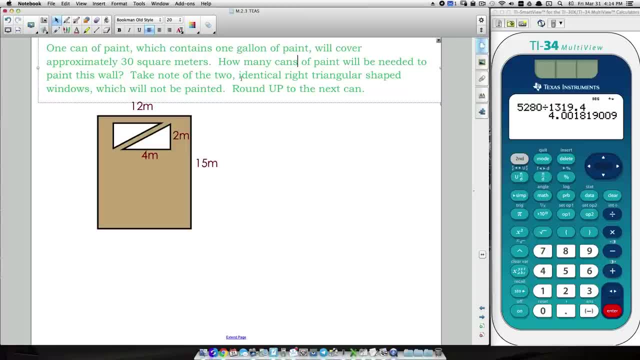 many cans of paint will be needed to paint this wall? Take note of the two identical right triangular shaped windows which will not be painted round up to the nearest cans. Notice I changed my little word there to can. Well, lucky for us, you know you have to be. 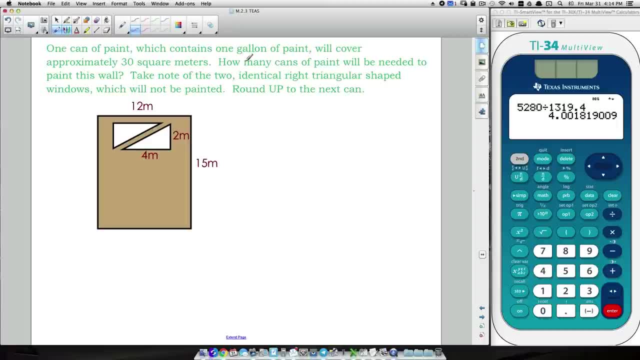 careful when you read it. But one can of paint is one gallon of paint. Okay, So the gallons are not even really that important here, because we're trying to figure out how many cans. But you know, you go buy a can of paint, it is, I think, most time they come in around. 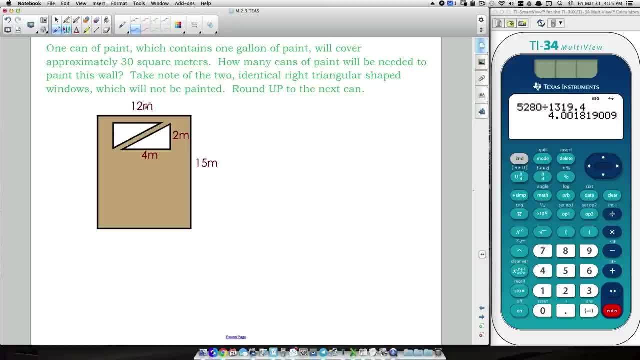 a gallon. I mean you can get pint sized ones and stuff like that as well, And everything's in meters. So we're trying to figure out: okay, 30 square meters- meters- we don't have to do any conversions here. That's great. Well, we're not gonna paint the windows, These are. 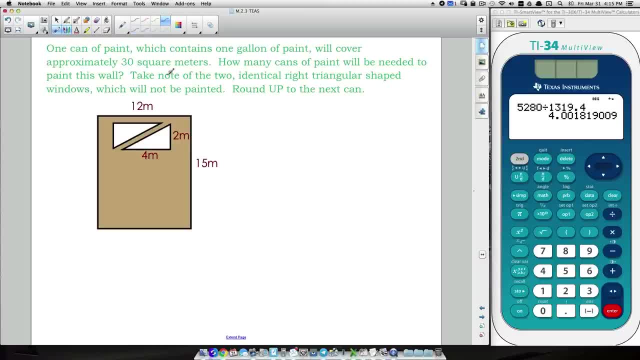 some weird shaped windows. I'm gonna give you a shortcut right here in a second, And maybe you already see it, But I'm gonna go ahead and talk about this. We want to take the area of the rectangle, So the area of our rectangle is going to be length times. 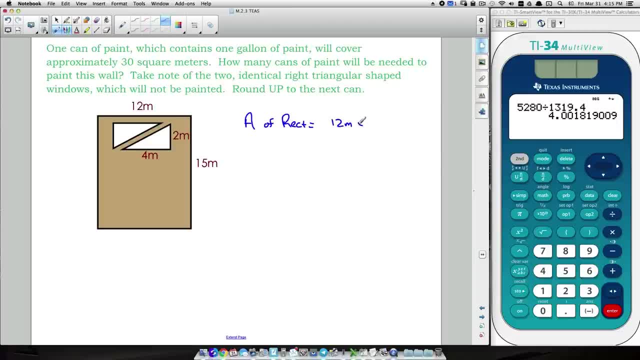 width. So 12 times 15.. So 12 meters times 15 meters, All right, And then just don't forget when, when you're multiplying these, it's always going to be in square units. So we're looking at 180 square meters. Okay, now this would be. 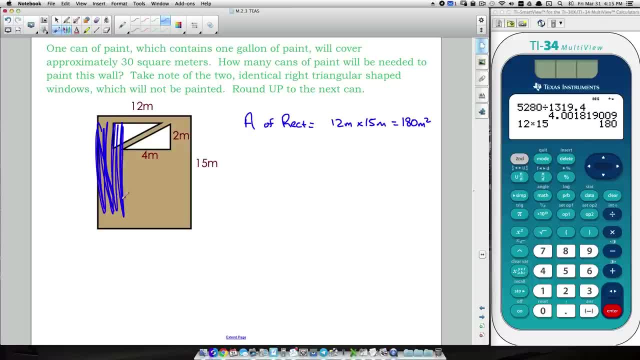 the number of square meters, if we painted the whole entire wall like that, the whole thing. Well, really, we don't want to paint these windows, So we want to kind of come back in here. we want to take that off- You don't want to paint it- and then go back and 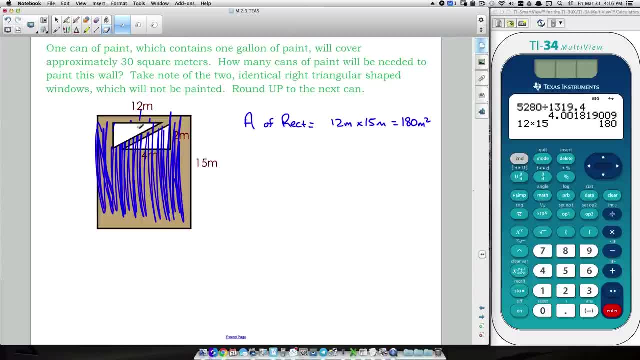 unpaint it, right, But really we're not painting that, So we're not going to paint that area of the wall. Notice, I said area And we're not gonna paint this area right here either, Right? So really, what we're going to do if these are identical triangles? 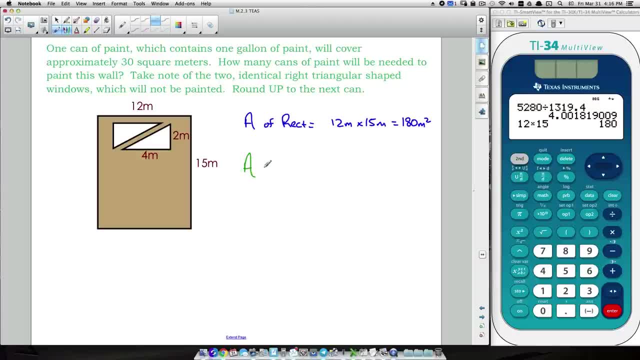 which they are. I'm gonna take the area of one triangle, and I haven't mentioned the triangle formula yet. But the area of a triangle is one half times the base, times the height. Well, which one's the base, Which one's the height? It does not matter, since we have a. 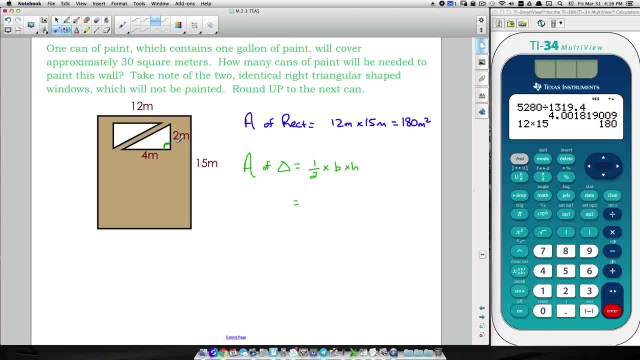 right triangle And I think for the most part you're going to be dealing with right triangles on the tease test. If not, you will probably be given the height or the base or something like that, But here at the base we can call that four. So one half times four meters. 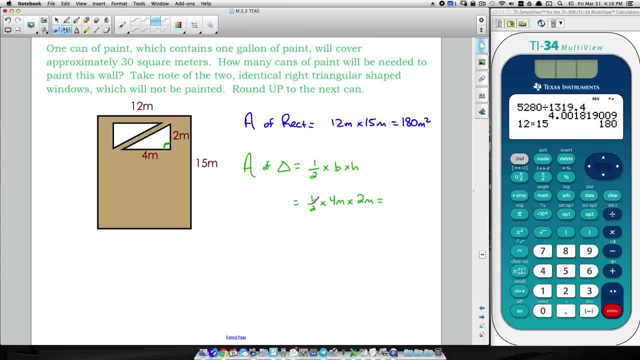 that's our base of two meters. So let's multiply this Four times two is eight, And then let's take half of eight, So half of eight is four square meters. Now this is the area of one triangle. Notice, we have two. 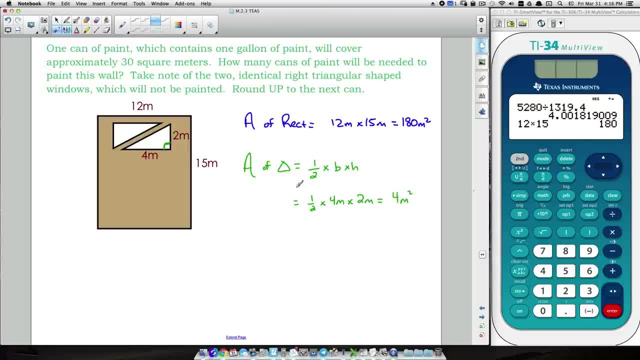 triangles. right, That's just the area of that one. Well, this triangle is identical, So we're just going to double this area, And we don't say times two square meters, We just double it, multiply it by two. So really the area of those two triangles together is going to be eight square. 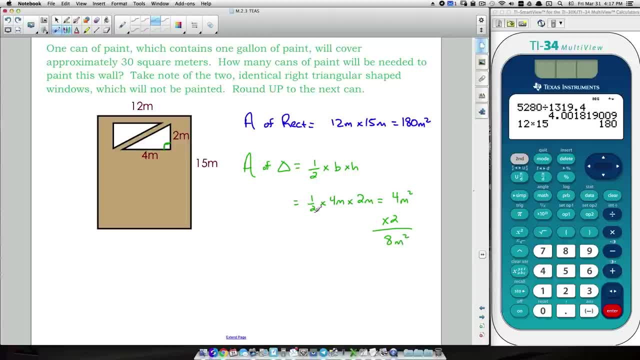 meters. Well, here is your shortcut. Okay, If we were to take these two triangles now, we can't do this in real life, but what I'm going to do is I'm going to take this triangle right here and I'm just going to drag it like that. What type of shape do we have? It's a rectangle, right? What's? 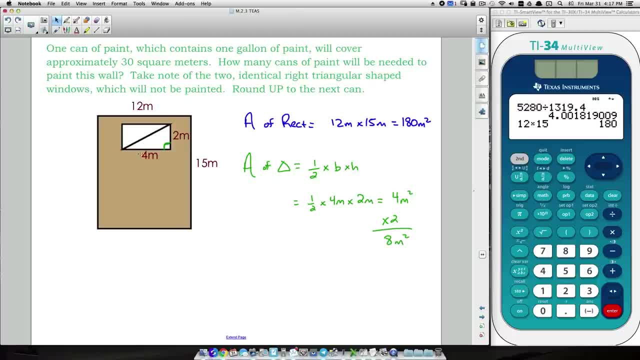 the area of a rectangle, Length times width, four times two. So really, even though we have two separate shapes, we can think of it as being one rectangle. That's where the area of a triangle comes from. Well, that, and a parallelogram, but nonetheless, look the area of this shape now. 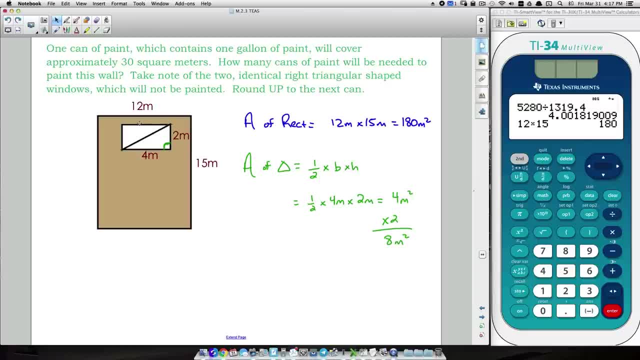 this rectangle, it's going to be four times two, which is eight Boom. It's the same exact answer, But again we have a weird window here. So, uh, I mean, most people probably are going to look at that Most. 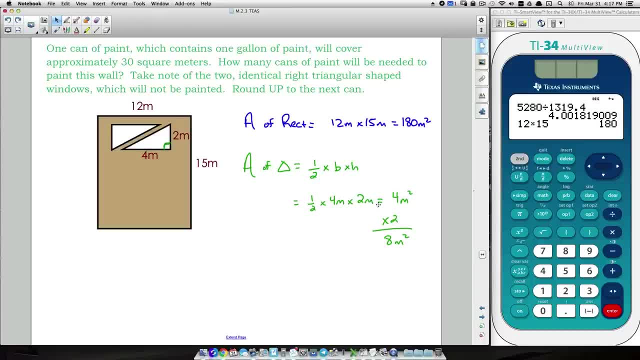 people probably are going to look at this and say, Hey, I need to find the area of this triangle. Got it, I got two of them, So we double it. but I want to go ahead and show that shortcut to you. So what do we do here? Remember how I colored everything in while I go? then I took away this. 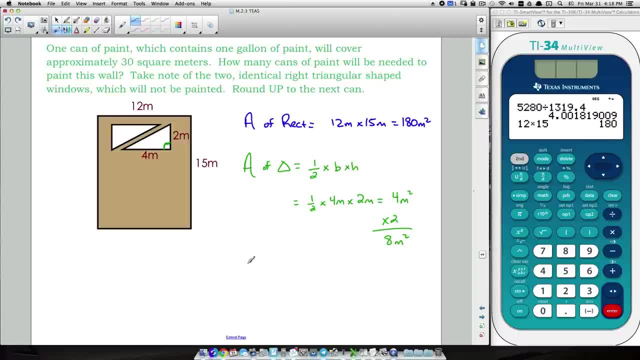 part and I took away that part. Well notice, I said took away. So, um, the the area to be to be painted, what area do we want to paint? We don't want to paint the full rectangle, So we're. 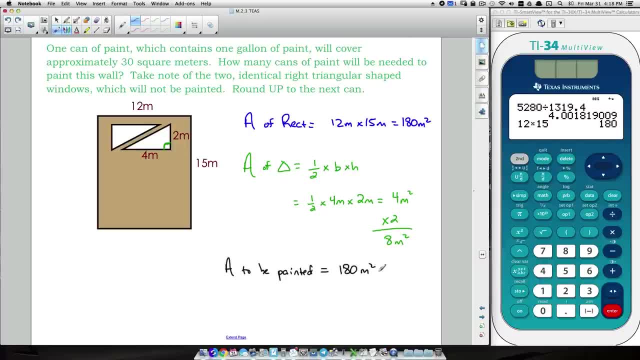 going to take that 180 square meters, and we don't want to paint the two windows, So we're going to subtract those eight square meters. Therefore, we're left with 172 square meters to paint. All right, So how many cans of paint do we need? Well, let's just uh, figure this out. 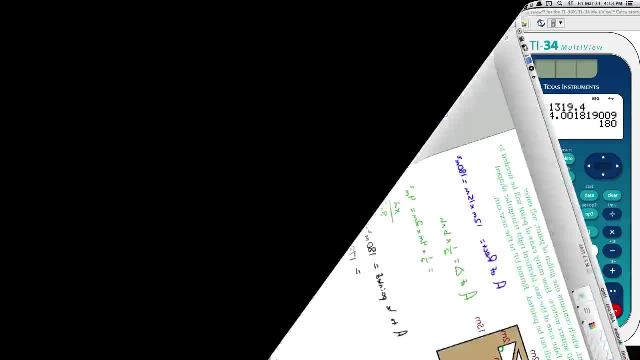 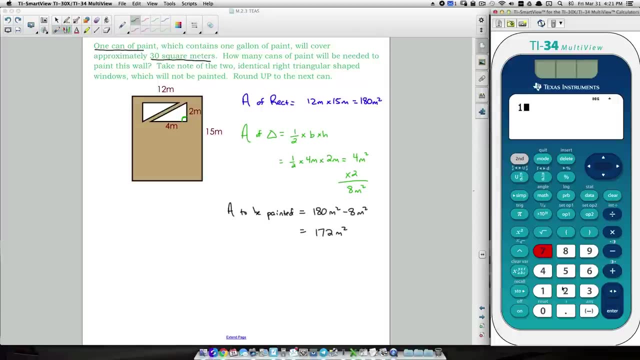 One way you can do it is: you can just divide by 30 and you're done. And let me go ahead and show that to you. Um, we, we can take this area that we want to paint, the, we take the 172 and we can divide by. 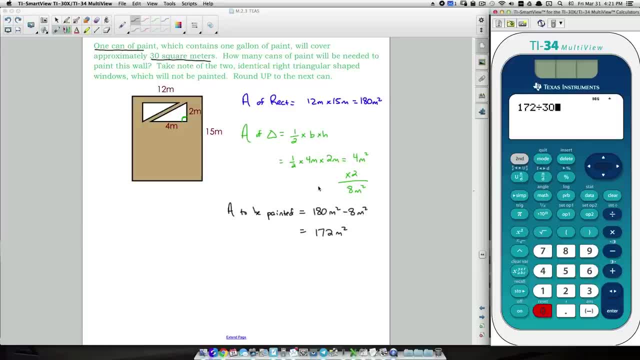 30, because, uh, we have 172 square meters. We can divide it up into 30 square meter sections, if you will, And that's going to tell us how many cans we need. Uh, so, uh, six cans of paint. 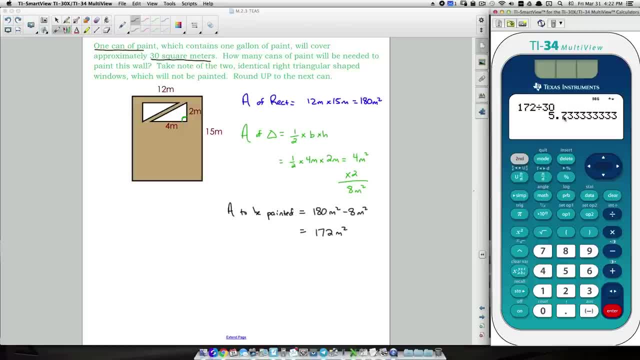 you know five cans of paint wouldn't cover it. Even if this was like 5.2, you would still want to round up, because you can't buy 5.2 cans of paint unless you went and got you know, one big can of paint and you got a little pint sample sizes, which 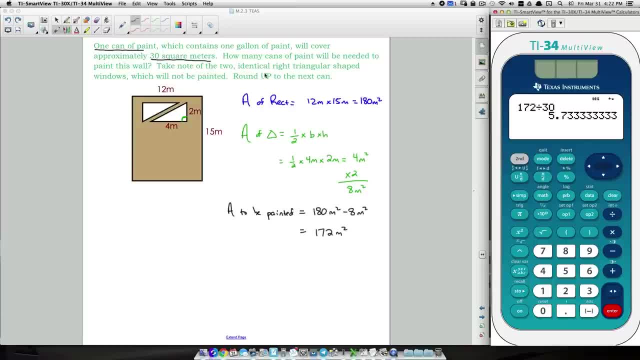 uh, everybody does. but it just says here in this problem, round up. regardless of our answer, we would round up, But here clearly we see we're going to round up to six. So watch this. We're going to get this same answer by taking a slightly longer approach, but probably a better to. 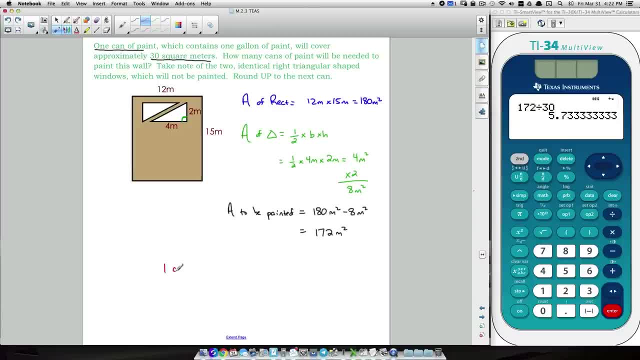 understand approach using a proportion. Well, what do we know? We know that one can of paint covers 30 square meters. So one can of paint, 30 square meters, equals X cans of paint. Notice, I'm putting cans, cans, And then at the bottom, um, we want to figure out how many cans. 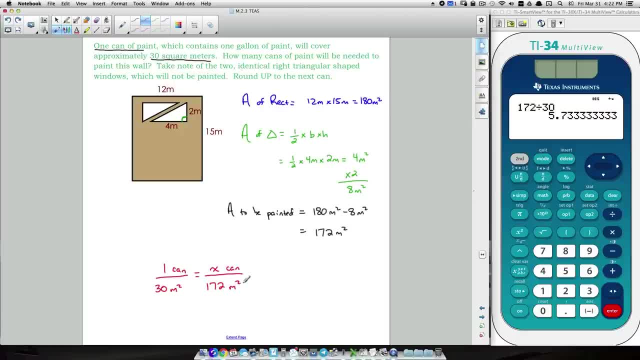 we'll cover 172 square meters. Well, if you solve this proportion, you will see that you take one times 172, which is 172.. And then what are we going to divide by the number getting multiplied by X? and notice, I am typing in the exact same thing as what I did up here. That was a shortcut.